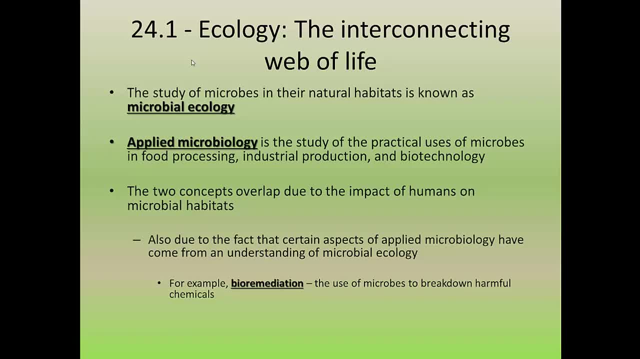 fit into those. So there's microbial ecology, there's ecology as a whole, and then this relates in a lot of ways, especially from a microbial sense, to applied microbiology. So we'll define ecology here in just a minute. but from a microbial standpoint it's really the study of microbes in 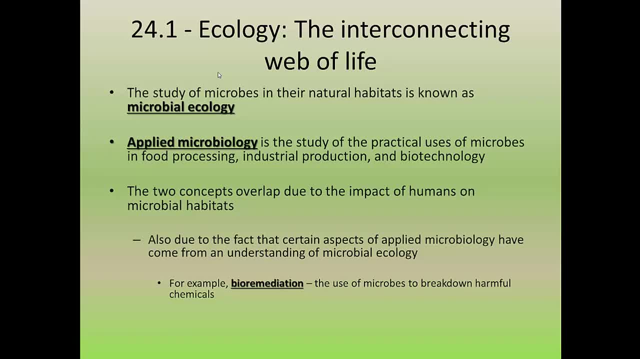 their natural habitat. It's kind of a simple way of looking at it. Now, this relates to a different topic called applied microbiology, in which you're using microbes for commercial and industrial processes, Things like you know. an example would be the production of antibiotics, Cheese manufacturing. is a big topic in microbiology, So it's a big topic in microbiology. So it's a big topic in microbiology. It's a big topic in microbiology, So it's a big topic in microbiology. So it's a big topic in microbiology. 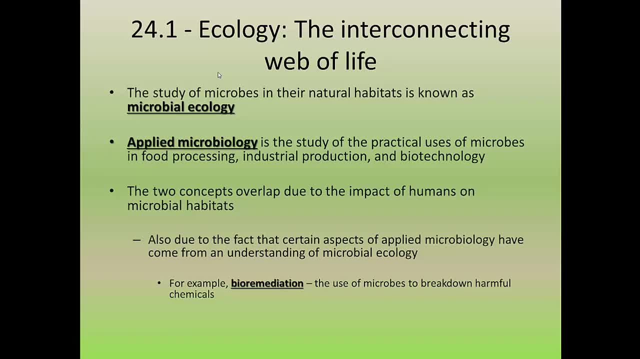 Is done using microbes, for another example. and another one would be like alcohol fermentation, So insulin production. We talked about genetic engineering. so these are all examples of applied microbiology And the two overlap in a lot of ways- not not in every way, but because a lot of times you're taking what happens in the environment and you're applying. 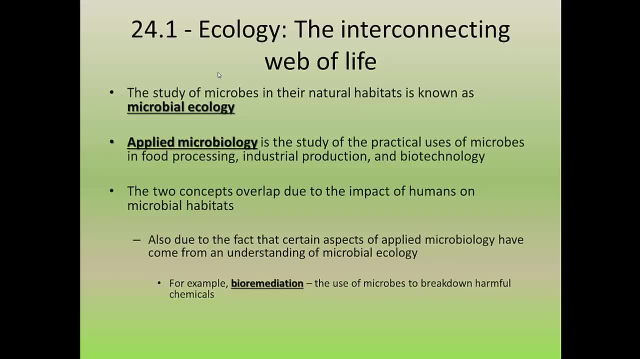 that to an industrial or commercial process. So one example would like penicillin, which comes from a natural fungi. Another example I have listed here is referred to as bioremediation. What that is is a process in which you're using microbes to clean up harmful chemicals and substances. It turns out 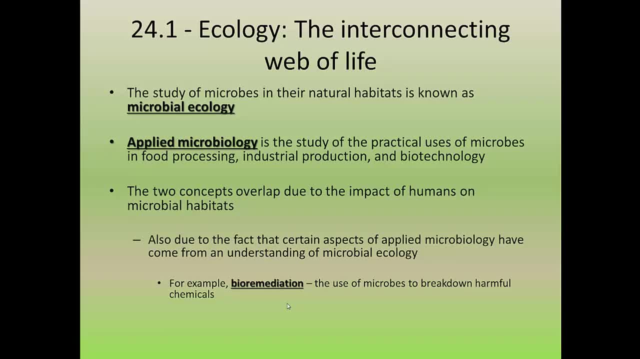 that microbes can break down almost any kind of substance that is found, And what's even more interesting is not only can they break down the naturally occurring substances- things that Mother Nature produces automatically- but it turns out there's lots of examples that have been shown that they can actually. 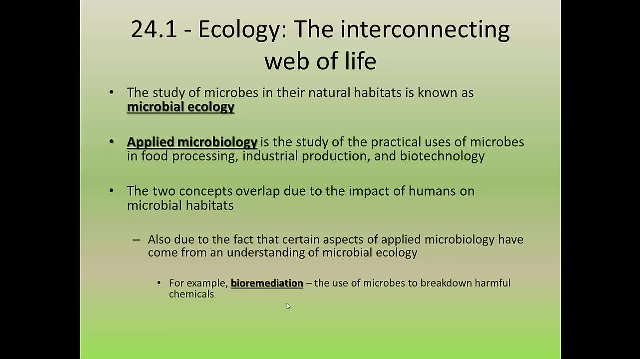 break down totally synthetic chemicals that are created by humans, that aren't naturally found. So it's almost like they're adapting on the fly. as we create new chemicals and new synthetic compounds, There are microbes that appear to pop up or adapt in a way that they can start to break those down. 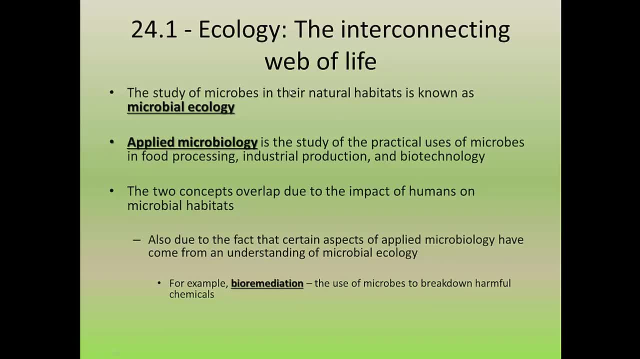 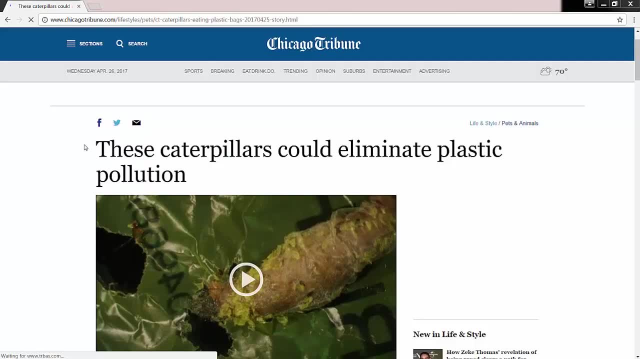 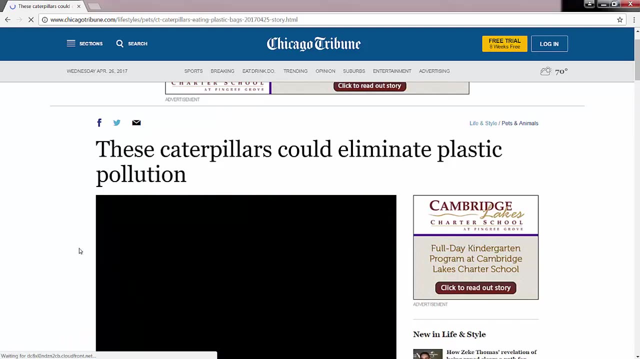 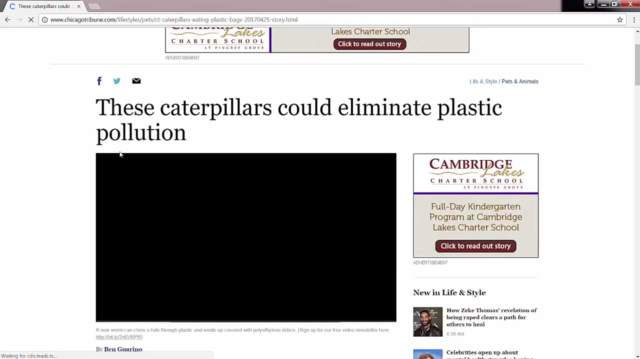 I'll give you a modern example here. This is April 2017.. This has just been in the news here, just recently. Let me pull it up real quick. So this particular article is coming from the Chicago Tribune, But there are lots of articles like it. Oh my goodness, There's lots of articles like it. So this 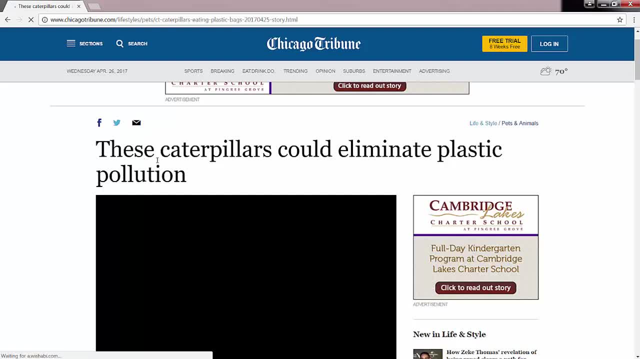 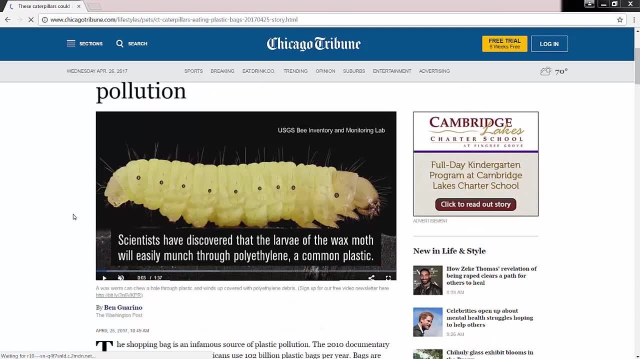 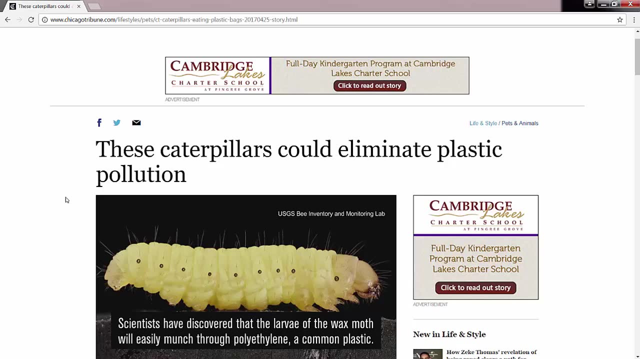 is just one example here, And what it's talking about is that caterpillars are being found to degrade and break down plastic. These commercials here. So caterpillars are being found to naturally break down plastics, which is odd because it's always been stated that nothing could. 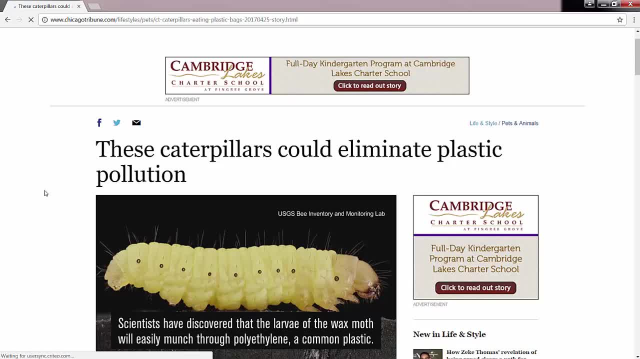 break down plastic. If you follow some of the environmental policies and concerns, one of the big issues is plastic. It doesn't in theory really Some people say it never breaks down It does. eventually It takes like a hundred years or more to break down, But it turns out these caterpillars actually eat it and 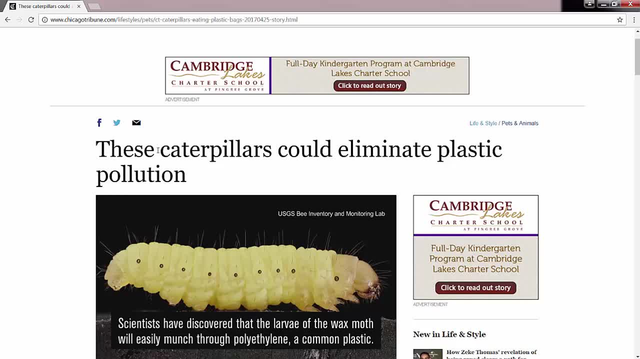 they can break it down into their stomach. they might be thinking: well, that's, how is that related to microbes? well, no one knows for sure yet, but most likely it's a combination of what the caterpillar is doing and also the microbes in its gut. now, that is somewhat of an assumption, because no one knows that for sure. 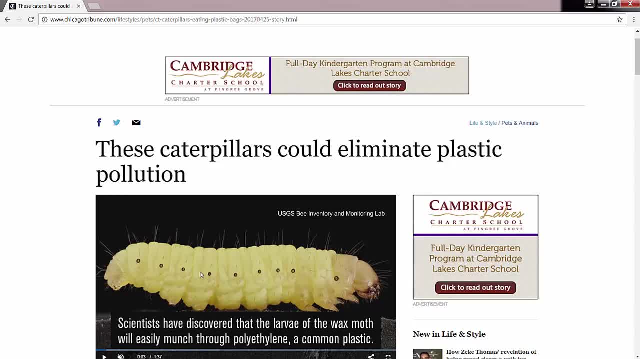 but in a lot of cases you have symbiotic relationships. it's like you know i have gut bacteria that help us digest food. uh, it's assumed that that's probably what's happening here with these caterpillars, because there's so many associations like that in nature, so that may. 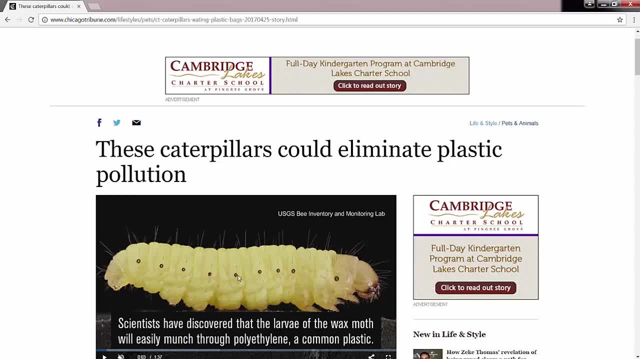 not be the case, but probably so. it's probably a combination of what the caterpillar does in combination with the bacteria. so the next step for these researchers is to try and extract the enzymes that come from either the caterpillar or from the microbes and see if they can use that. 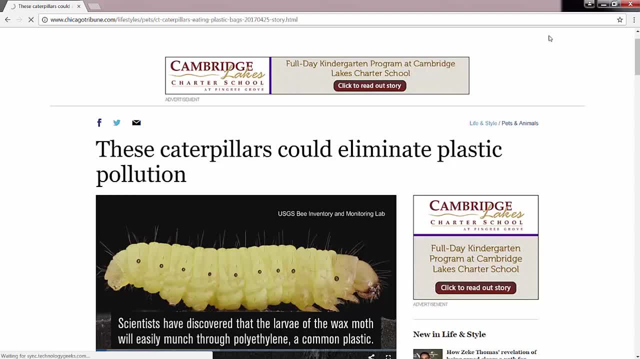 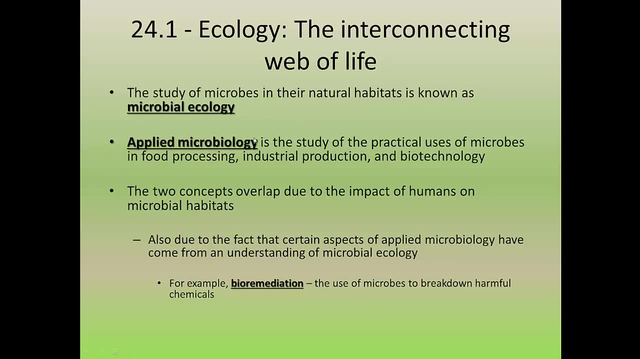 in an industrial process. so basically recreate that enzyme on a larger scale and be able to make a chemical or a product that you could use to break down plastic. so look for that to come in, hopefully in the coming years. probably take a while, but that could be a major breakthrough when. 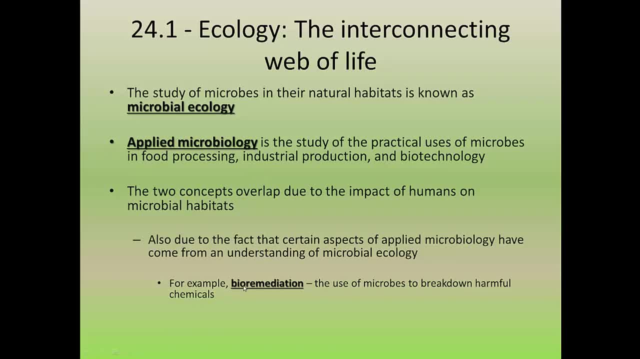 it comes to you plastic pollution problems. so that's an example, kind of like an example of bioremediation. assuming it is microbes that are going to be part of that, then you could consider bioremediation. even if it is the caterpillar, it's still pretty much the same thing. so by learning what the 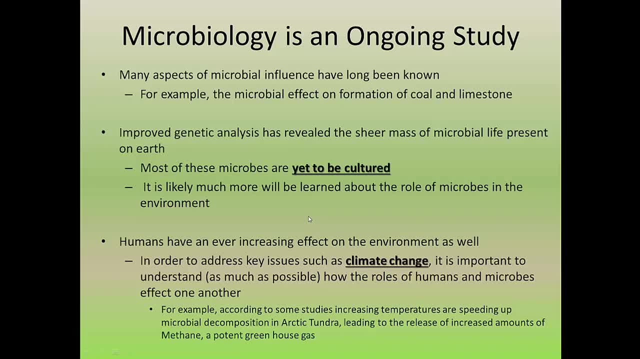 caterpillar is doing, and you can then apply that at an industrial level. so lots of other examples. a couple years ago they found a microbe that could break down styrofoam as well. so now, like micro in other aspects of human microbiology, in- uh, in research, it's true, also in an environment, micro that scientists don't really know that much. 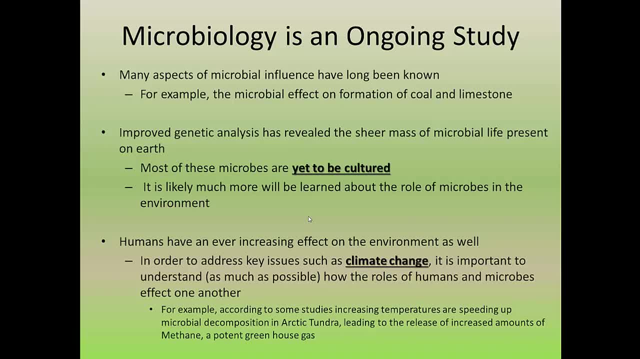 because of the limited cultural, cultural ability- uh, culture ability- to grow these microbes in the lab under artificial conditions. so, as a result, most microbes are yet to be cultured. so remember the number: it's about one percent that's estimated to actually be cultured at this point. so in theory, 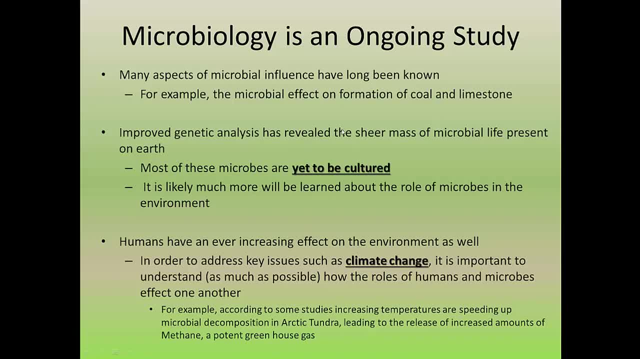 99 percent of what's out there really hasn't even been explored much, let much, much less thoroughly researched. so there's a lot to know now. there's a lot of ways that that research could impact our lives, but one of the more pertinent and maybe maybe more relevant examples- certainly one. 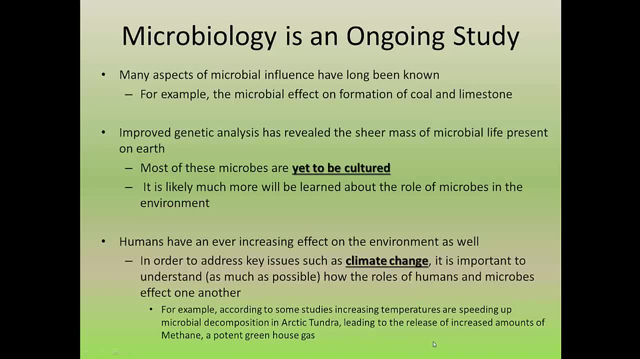 that's discussed more than others. it has to do with climate change, you might wonder. well, how do microbes have anything to do with climate change? well, they may not have as much to do with humans, as much to do as humans, which humans certainly have the biggest impact. but it turns out that microbes 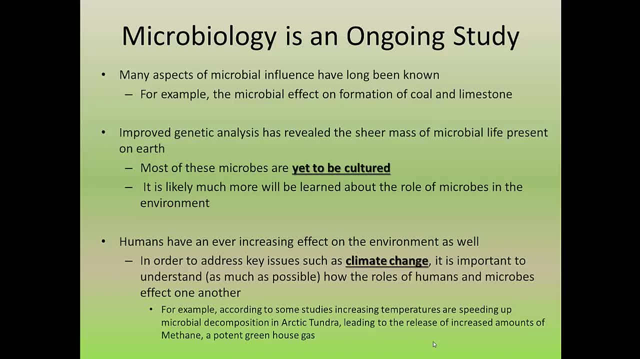 can actually have an impact on the climate, especially in combination with a warming temperature. so it's just one example researchers have found in Arctic tundra, especially in the northern parts of Russia, they've got lots of permafrost. it's an area where most of the year it's it's frozen and the ground is. 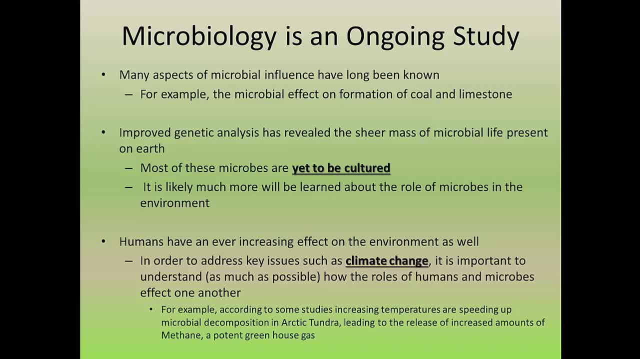 relatively relatively low, and metabolic activity at those cold temperatures not a whole lot of metabolic activity is happening for most organisms and what they're finding is that, as the temperature is warming just ever so slightly, there's more metabolic activity when it comes to microbes, and some of those microbes release a chemical or a. 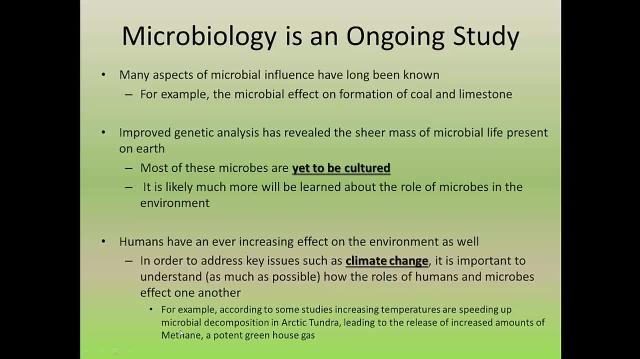 compound called methane, which is a potent greenhouse gas that we'll talk about in part two. so methane is a is a greenhouse gas like co2, and so what they're finding is, as the level of the temperature goes up, metabolic activity goes up and, as a result, more methane is released. so the big question, or the big issue really is: 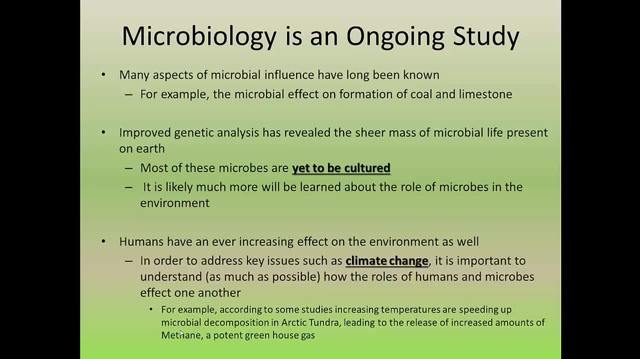 are we affecting climate change even more by affecting the way microbes naturally release chemicals like methane? so there's just a slight connection there. could that could turn out to be negligible, the effect may have no real impact, or it could turn out to be a big impact, and that's what we're looking at. 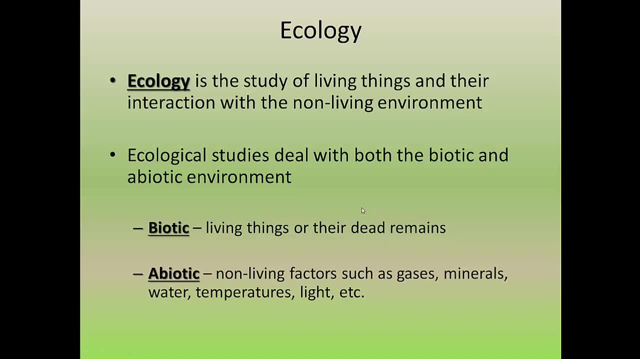 so there's just a slight connection there. could that could turn out to be negligible, the effect may have no real impact, or it could turn out to be a big impact and no one really knows. and that's kind of point is that no one really knows. but there is at least a potential impact there, and so it's. 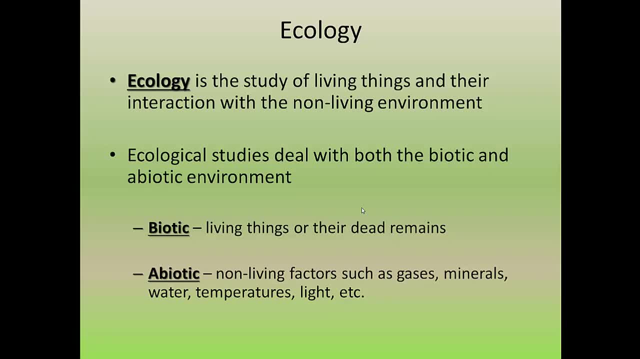 something that's worth studying. so these are examples of how more research can help us understand that interaction between microbes in the environment and then in a place like climate change, just a big issue, how that might impact us in the future. so ecology- there's microbial ecology isn't really ecology, is its own. 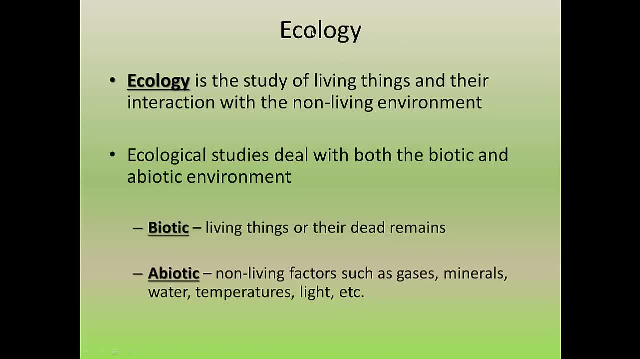 field. it's really kind of a subfield in the sciences related to biology, but but actually somewhat of a secondary or, excuse me, a separate field. And so what ecology is? it's looking at the study of the living and the non-living environment. 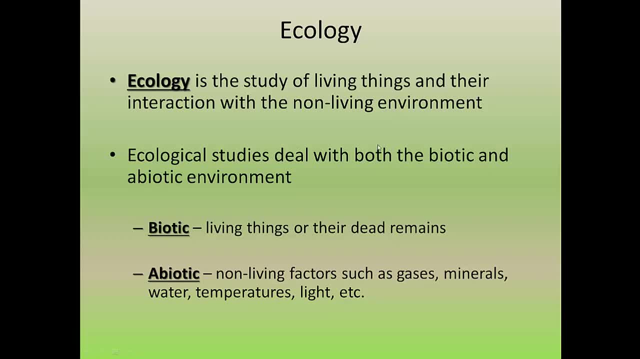 So the study of living things and their interaction with the non-living environment. So, when it comes to these ecological studies, you have what's called, you have what are called biotic components, and these are both the living things and or their dead remains or anything associated with them. 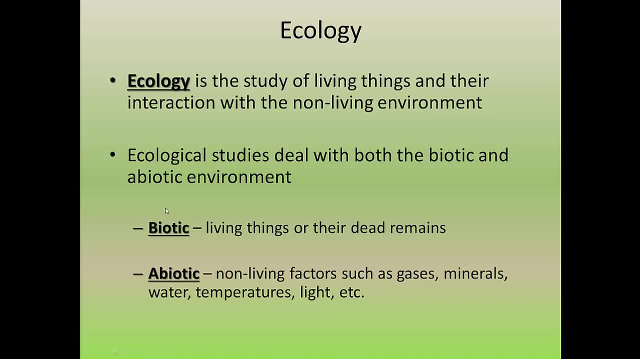 such as like fecal matter or waste. So biotic is not just what's alive at this moment, but also what has been alive at some point or comes from a living thing. Abiotic would be any non-living factor that has never had a living component to it. 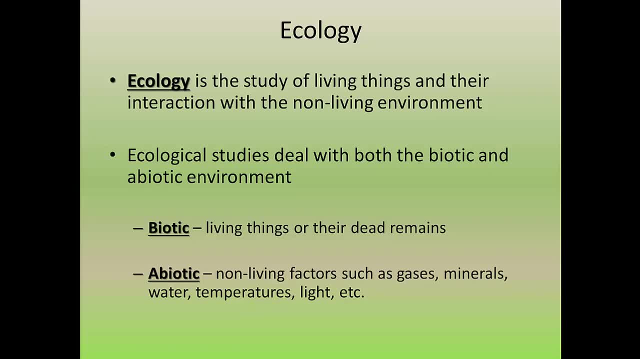 or never had a life property, such as the gas in the air, the minerals in the soil, the water, temperatures, things like that, the light. These have never been alive, and so they're considered abiotic. So even something dead would be considered biotic. 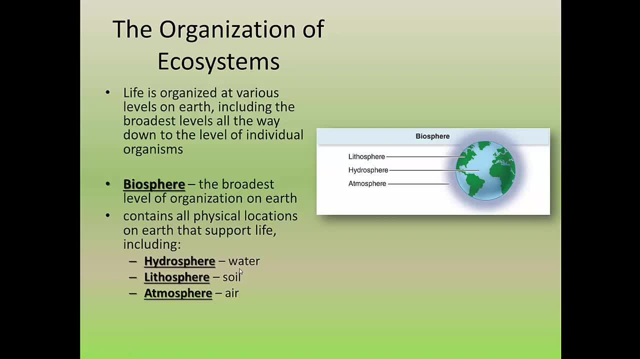 So that's ecology. So ecology, you know again, can look at lots of different areas, but microbial ecology is one of those areas where you're looking at just the living microbes in their non-living environment. So next we'll talk about ecology, some of these, one of at least a couple of the key aspects of ecology. 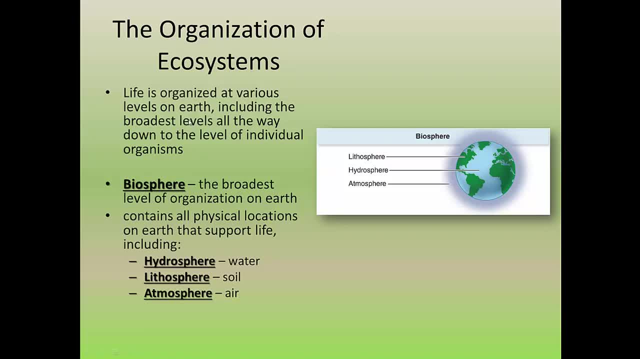 starting with some of the organization aspects. organizational aspects, So this would apply to pretty much all creatures- It's in all aspects of an ecosystem- but also microbes as well, So it will fit in specific microbial-related aspects as we go here. So when we look at an ecosystem, we can look at it from different levels. 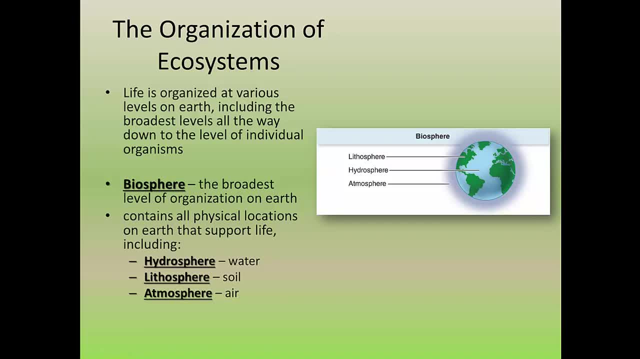 starting with the broadest level all the way down to the most specific. So with the broadest level we have basically the entire planet as our broadest level of an ecosystem. We call this the biosphere. So the biosphere is the ecosystem we call planet Earth. 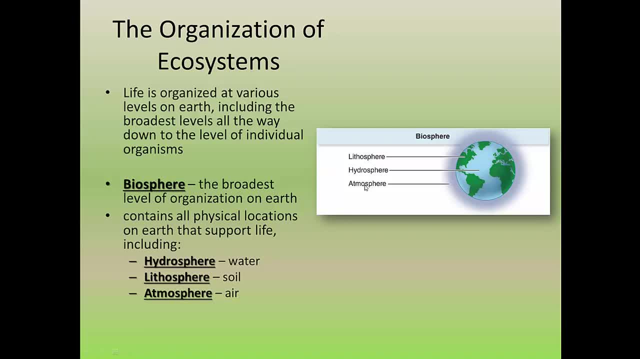 Now we can then break that. We can then break that down into several compartments to help analyze some of the key aspects separately. So, for example, we can look at the hydrosphere, which is the water. We can look at the atmosphere, which, as we know, is the air. 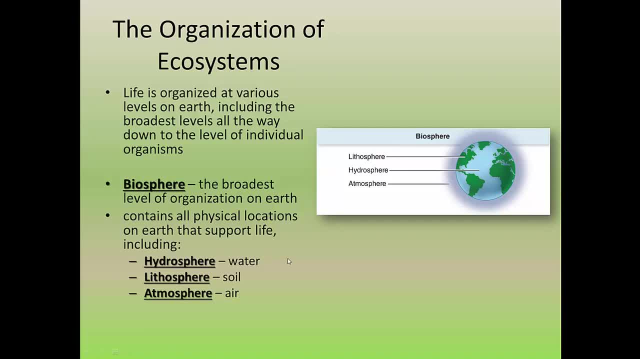 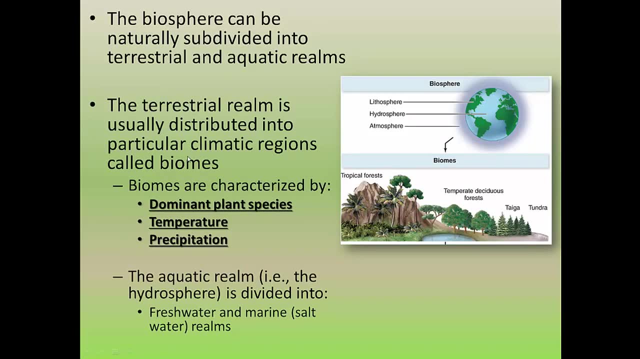 And then there's what's called the lithosphere, which is the soil. So those are the least three major compartments of the Earth. Now, most life takes place within the terrestrial and aquatic realms, The atmosphere, the air. there's lots of living things in the air. 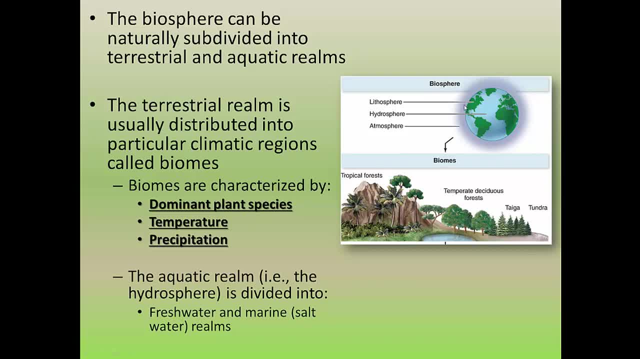 but they're more or less transient, meaning that they are just simply being moved from one area to the next. No organisms really habitate in the atmosphere, They're just moving through it. So when we look at life, we're really looking at life as it pertains to what we call the terrestrial on land. 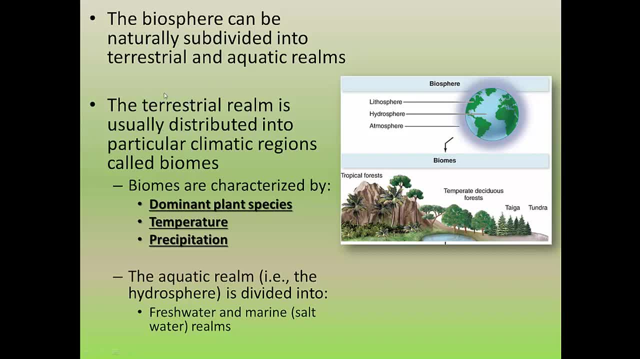 and then the aquatic in the water. Now terrestrial realms are a little easier to categorize in that they have specific characteristics to them, So we can break the terrestrial realm into regions, what we call biomes. So a biome is kind of a unique part of the terrestrial landscape. 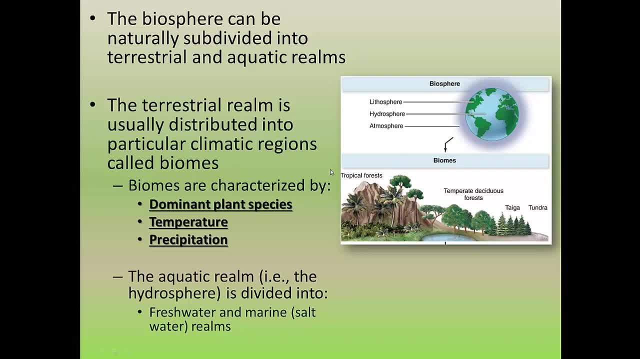 So examples would be like a tropical forest, That's a type of biome. like the rainforest, You have certain types of what are called deciduous forests. Taiga is like a northern forest. It's kind of a northern kind of largely dominated by pine trees kind of area. 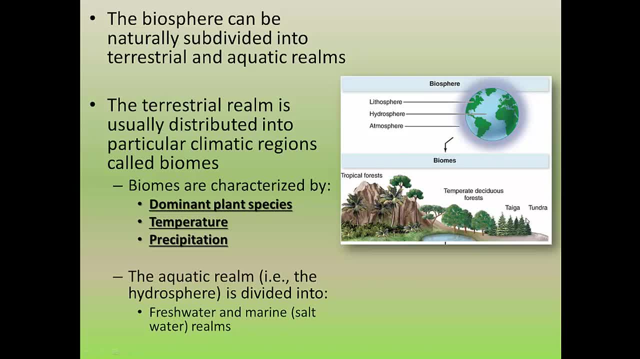 Chandra is kind of a lot of open, like another northern kind of cold, almost like a prairie grass kind of landscape that's in the northern part of the world. Desert would be another. So these are all just kind of general examples of a biome. 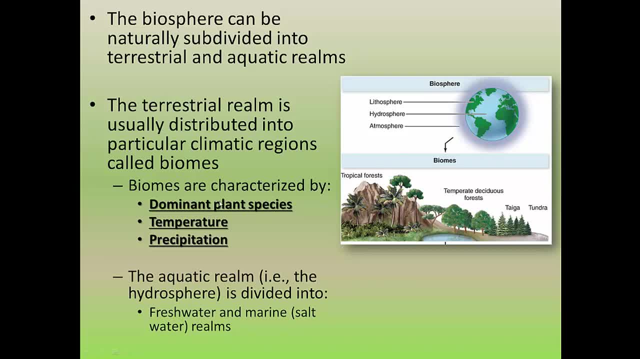 But what characterizes each are the types of dominant plant species, So each one tends to have a different type of plant. Tropical rainforest being, you know things like palm trees, for example, taiga being, things like pine trees, What are called gymnosperms. 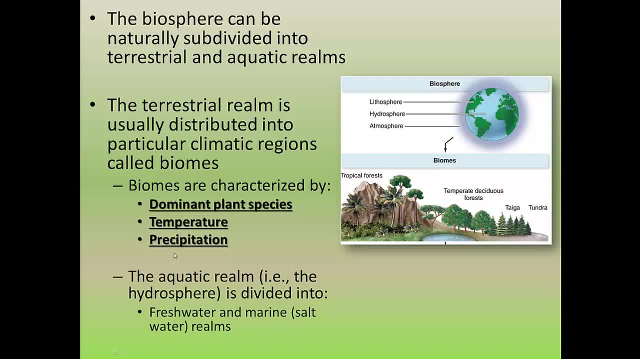 The temperature and then the rainfall precipitation. And temperature has a lot to do with the latitude. So as you move north or south from the equator temperatures tend to go down. So temperature is most stable here in the middle. goes down either direction away from the equator. 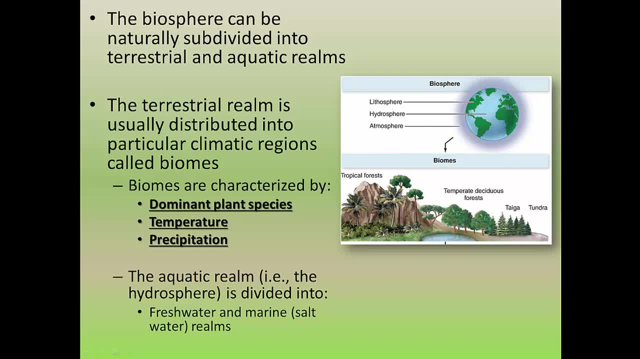 So the temperature then moving north or south, will affect the dominant plant species And to some extent. to some extent will affect the rainfall. Rainfall is typically heaviest right around the equator, So more sporadic, less consistent as you go north or south. 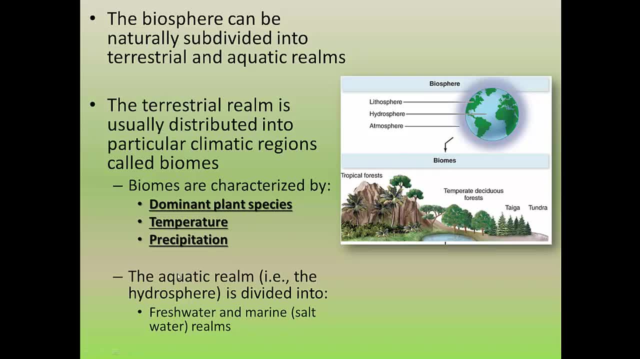 So all those things affect the landscape, and then we call it terrestrial biomes. The aquatic realm is a little harder to categorize, although you certainly could get into more detail there, But for for this discussion we just break it into freshwater and marine or saltwater realms. 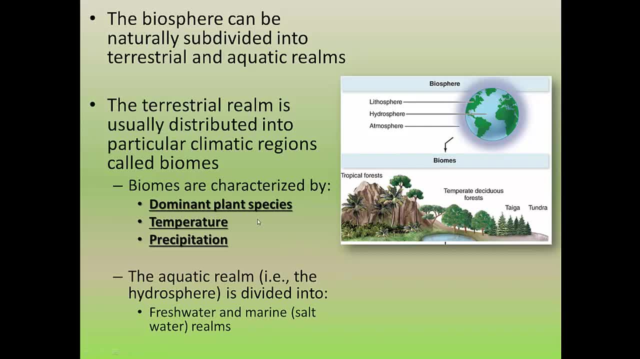 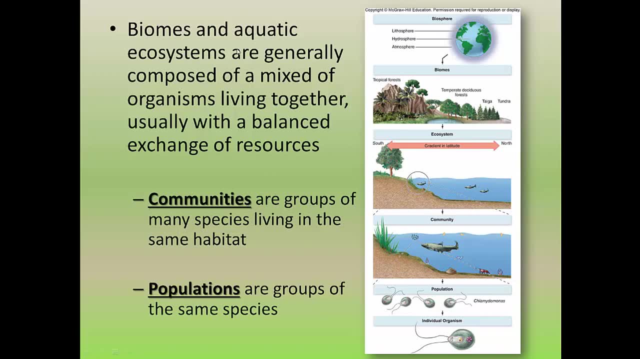 So you've pretty much got the ocean and all of its components, and then everything We would consider freshwater, like the Great Lakes, for example. Now, each terrestrial biome or aquatic realm or ecosystem, those are more or less the locations, based on the plant species and the precipitation and temperature. 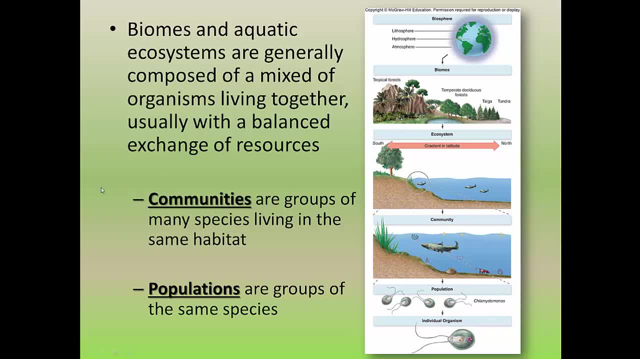 Within that then you have the communities of living organisms, go along with the plant species. So communities are basically your groups of living organisms All living within that particular biome or aquatic realm. So in Kansas, for example, we have a prairie grass type of biome and 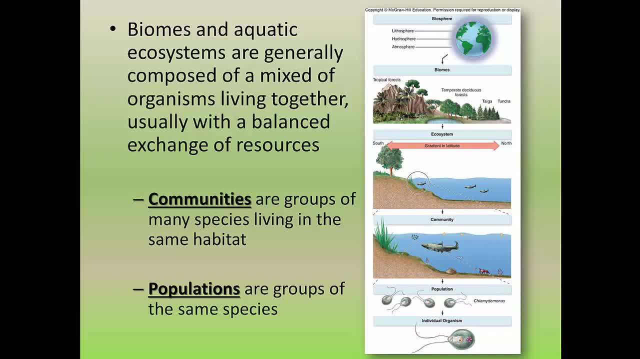 our communities are largely made up of, you know, things like rabbits and squirrels and birds, like robins and hawks and owls, and we've got certain types of insects and those types of communities are what we would consider kind of a prairie grass. 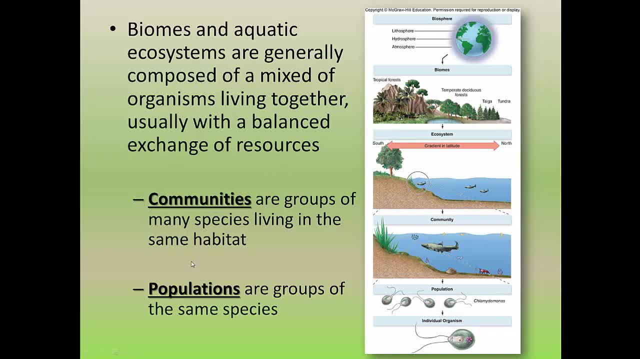 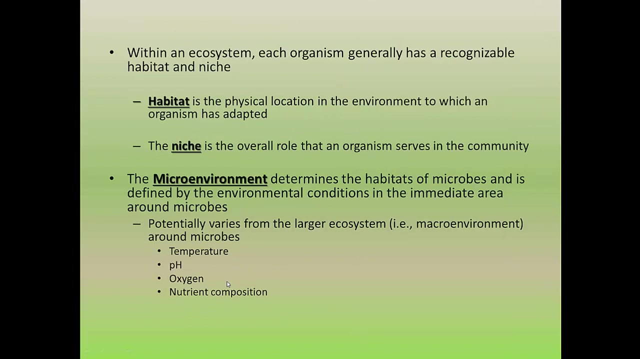 community Populations, then, would be looking at any one of those particular groups of organisms by itself. So the population of squirrels, the populations of red-tailed hawks, for example, All of these would be their own particular population. Within that population or, excuse me, within that ecosystem, then each member of a population has its own. 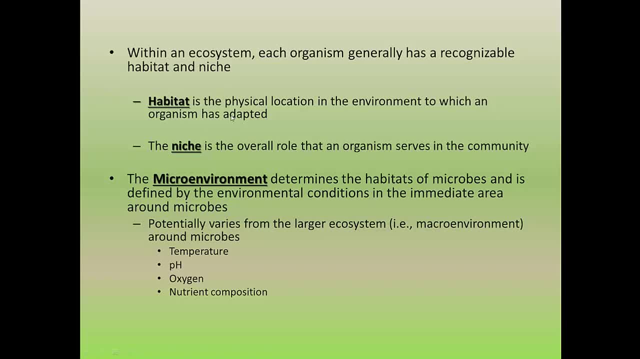 habitat. Now, usually a species kind of has its own type of habitat, but really each organism can have its own particular habitat in which it's a location that it's adapted to live in and survive. with them, The niche is the overall role that the organism plays. Sometimes that role is very obvious. 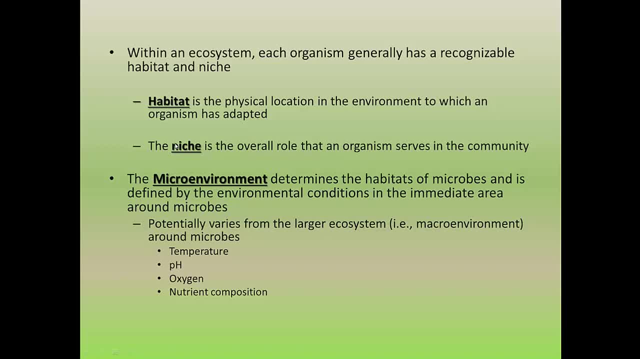 Some organisms. unfortunately for them, their role or their niche is to simply be a food source for other organisms. So this is the case for a lot of plants. So I'd say that's their only role. but one of their more obvious roles is that for plants, they feed other organisms. 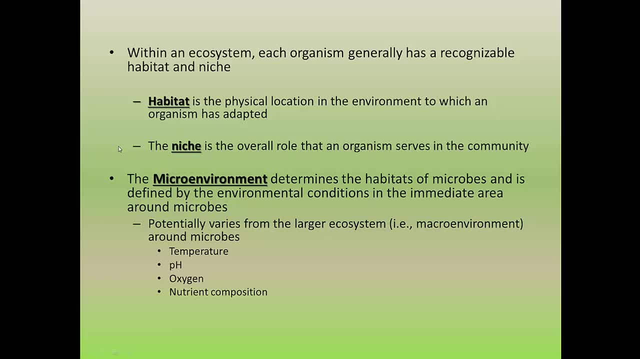 So that's the more obvious role. In some cases, the niche may be to lower the population of certain insects, like bats, for example. They feed off of things like mosquitoes and a big role that they play is to reduce mosquito populations. Now, there's lots of ways to look at a niche, So bats do more than just eat mosquitoes, for example. but a niche is kind of an. 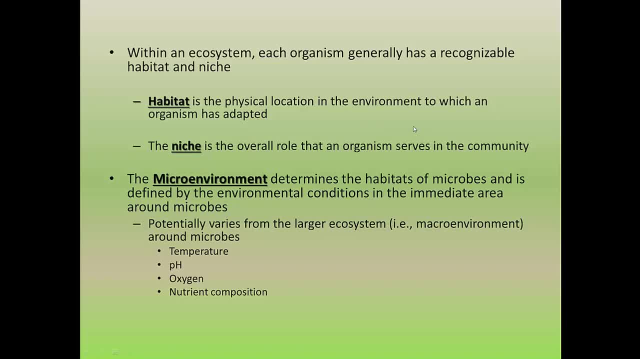 particular role that they might play in one capacity or another. Sometimes the role is more obvious, sometimes the role is less obvious, but that's the idea behind the niche. Now, when it comes to microbes in reference to the habitat, microbes are so small as we know. 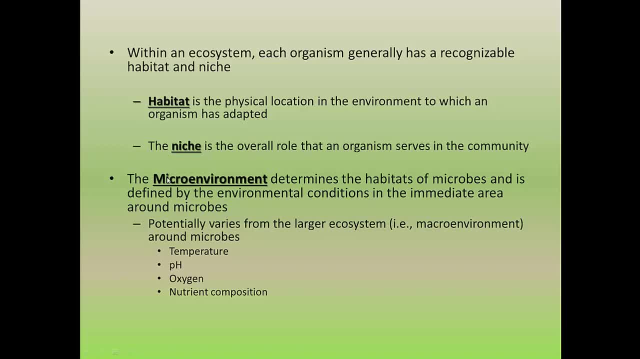 their habitat is what we often refer to as the microenvironment. The microenvironment is a very specific microscopic area in which they're found. Now, what's important to recognize about that is that the microenvironment can potentially vary dramatically from the larger ecosystem, what we call the macroenvironment around them. 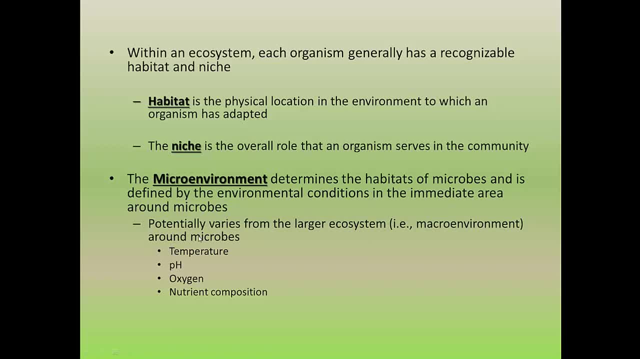 This is especially true when it comes to temperature, especially as you go deeper into the soil. so microbes in the soil, as you look from, say, the surface of the soil all the way down, you know as much as 20 feet or so. 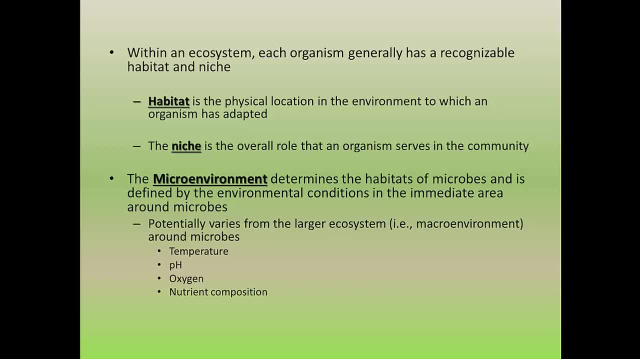 certainly just down to say, let's say, 6 feet. there's a significant gradation of different types of microbes with every so many inches as you go down in the soil, because as you go deeper the temperature decreases and, as a result, different microbes have adapted to those temperature changes. pH. 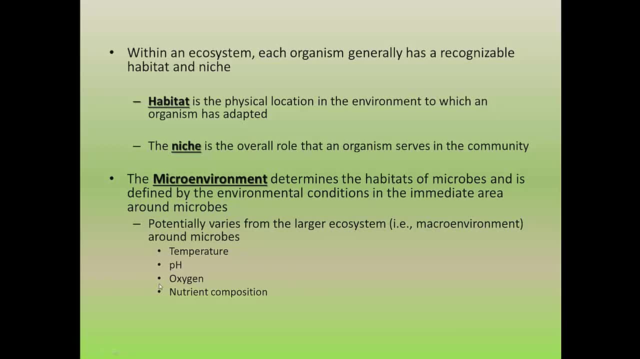 can change. oxygen definitely will change. oxygen goes down as you go lower into the soil, so that also affects microbes and then the nutrients can change as well. so you each, each area, might have a dominant type of kind of macro population of species, the larger species, but the micro environment and 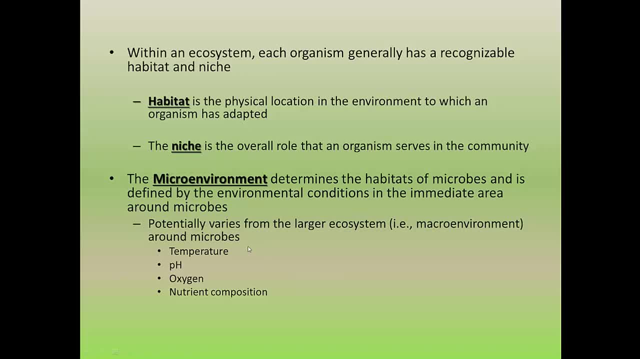 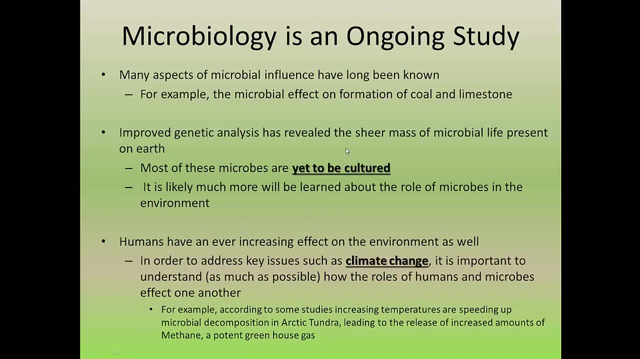 the micro microbial species can be dramatically different from one area to the next, and one of the things why that's important going back to this idea that it's an ongoing study. that means that if you want to study the microbes within an environment you don't have, you can't just look at the larger population. 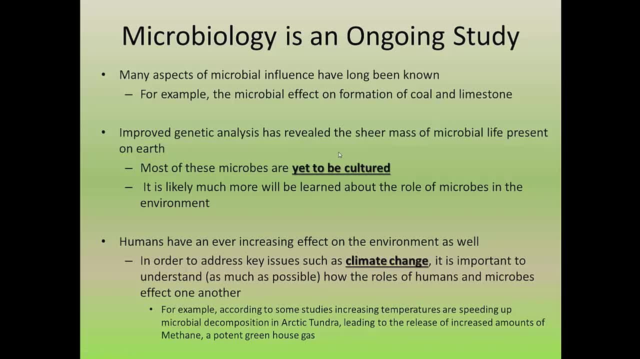 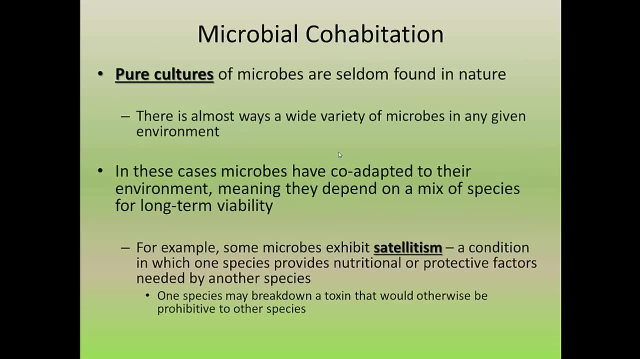 like you would some of the bigger species. you have to really look in every location, so many feet down in the soil, and I'm really that level of complexity you- it seems impossible that they would ever study every aspect of it. so I think- for from a realistic standpoint, there's so many different micro environments on 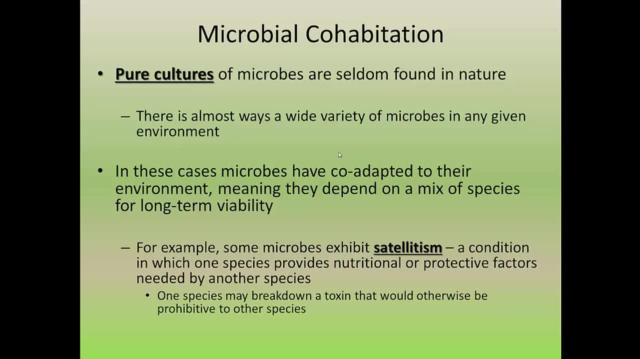 earth seem impossible that anybody could ever actually study all of them. so microbes are highly diverse. they come in all sorts of all sorts of forms, and every little square inch of the soil could theoretically be different from the next. so that's where the micro environment in the microbial species are. 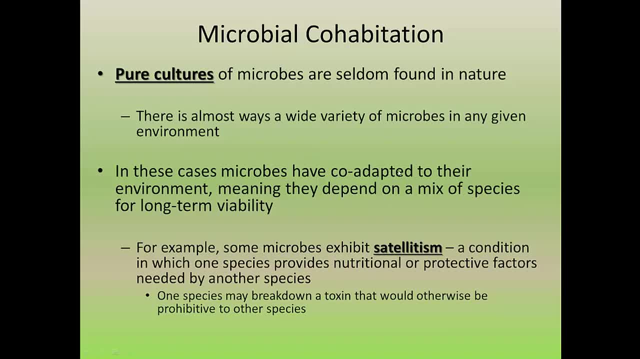 a little different from the larger groups around them. now one of the things that they have found consistently is that microbes never, or I should say hardly ever- there is an exception, hardly ever- or found what we call a pure culture, almost always a wide variety of them, and that's because microbes like 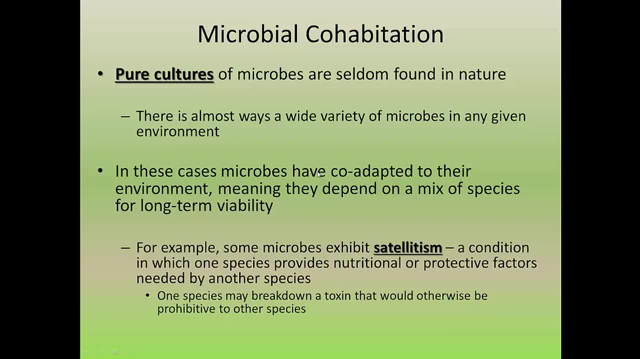 humans and like a lot of organisms, we are considered to be co-adapted or we co-habitate our environment. so that means that they depend microbes depend on other microbes around them for survival and sustenance. so we're kind of like humans: think about our own lives. for most of us we probably 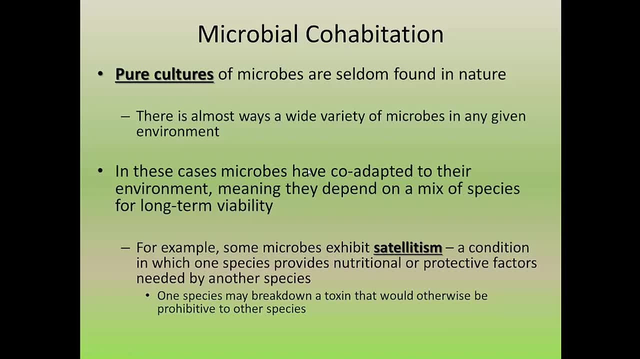 depend on our grocery stores for food. we probably depend on a gas station for transportation. we depend on a community for health care. we depend on a community for safety and protection. we depend on communities for things like insurance to cover us if accidents happen, so we don't do everything on our own, you know. 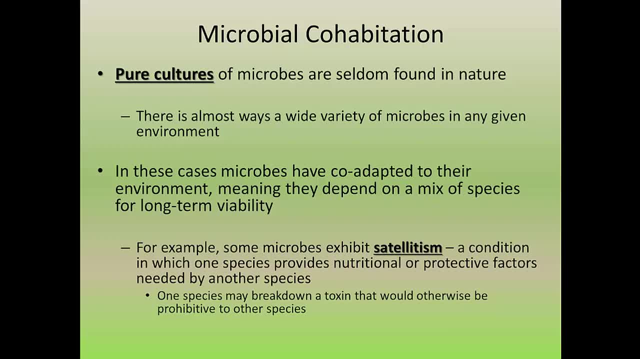 we, we largely take care of ourselves, but we we do depend on others for various different aspects. so imagine how much more difficult your life would be if you found yourself in the middle of an isolated Forest with no other species or no other human was around to assist you. you suddenly would. 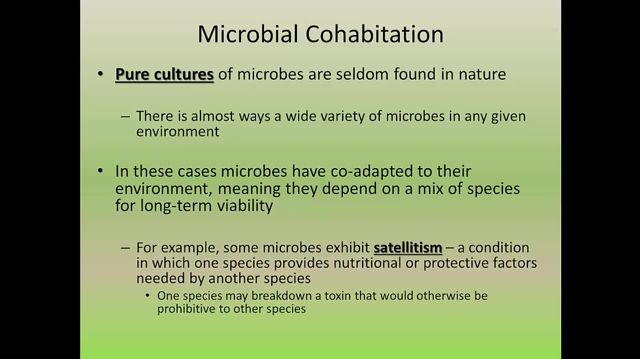 be 100 dependent upon yourself to create food, create shelter, find water and Etc. that'd be a difficult thing and a lot of us probably wouldn't make it. and so the same is true of microbes. they depend on other microbes around them, just just a less. 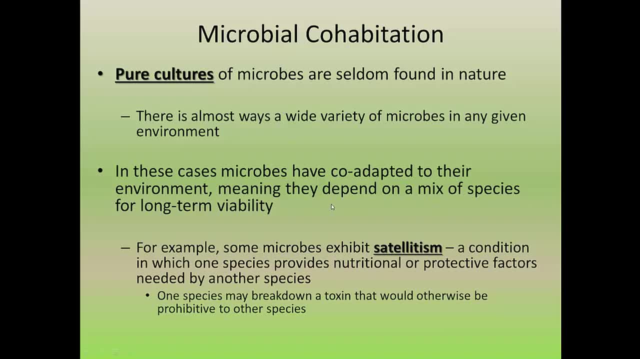 obvious ways. so, for example, the microbes are designed to to feed each other, so one microbe may produce a food product for another. it's kind of like one man's waste of another's treasure. uh, one microbe may expel a waste product that another microbe uses as a food source. 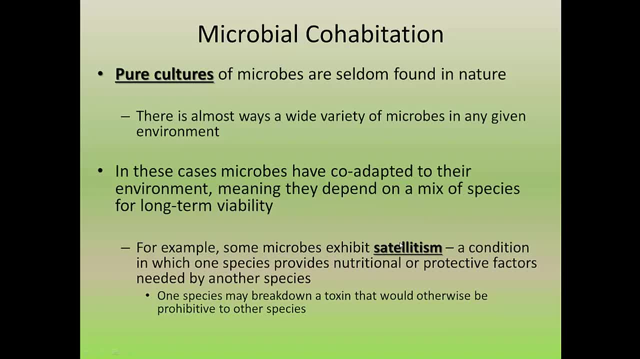 um, this is what we often refer to as uh satelliteism. it's a. it's a process in which one microbe provides a nutritional or protective factor needed by another. so what ends up happening is they end up kind of depending on other microbes around them, so in some examples, one species may actually break. 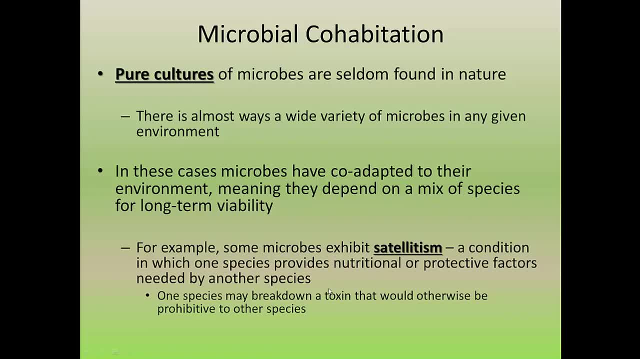 down a toxin that would otherwise be prohibitive to another species, so they kind of clear a safe zone, so to speak, for other microbes. and so this, once again, when you go back to the why we can't culture most microbes at least, why it's difficult, it's tough to replicate the natural environment. 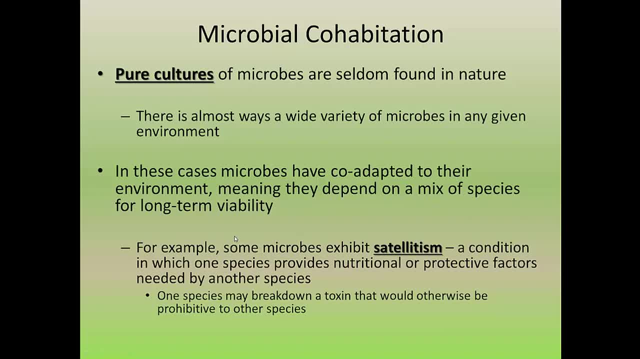 in a petri dish or in the lab, and so you have a lot of complex interactions that are normally happening and, if you recall from our lab, most microbes are grown in pure culture and so we're used to growing the species that do grow in isolation, but in nature that just doesn't really. 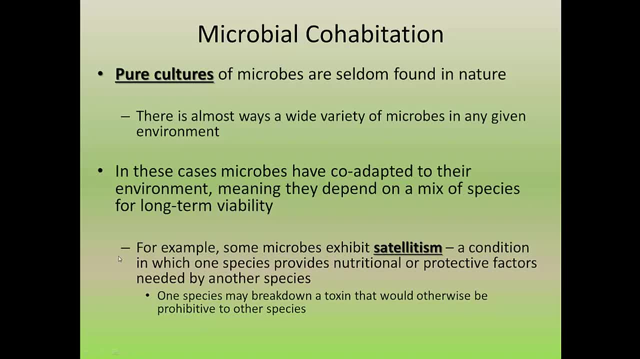 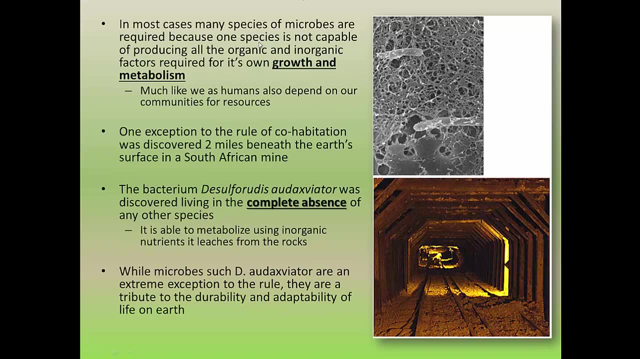 happen, and so the the trick of microbiologists, the trick that microbiologists are trying to accomplish now is to replicate this, these natural processes like satelliteism, to get microbes to work in conjunction in the lab, and that's just much easier said than done now. there are exceptions to every rule, and I put this exception here to give me an idea of just kind. 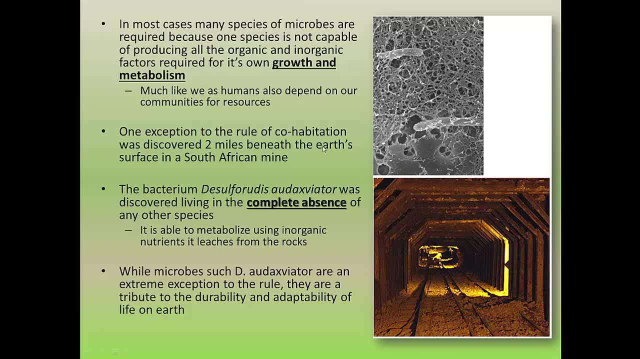 of how rare the exceptions are and kind of where you would find them, at least in this example. so there's a microbe- I'm not even going to say the name, but it's listed right here. this is the name of the species. they found this microbe actually growing as a pure culture, in isolation of any 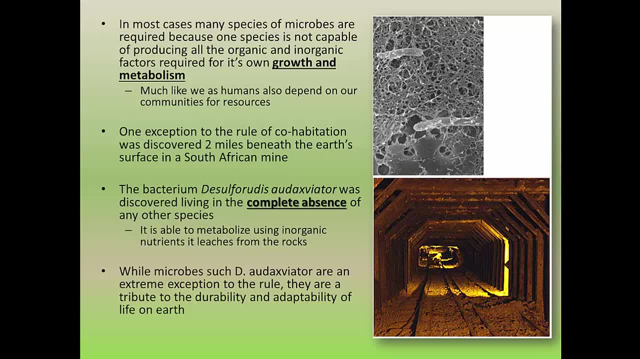 other species so there. so there are cases where this does happen. but where they found this, they found it two miles beneath the Earth's surface in a South African coal mine. so they had to go all the way beneath the surface and they- they already had the coal mine there and and some researchers went- 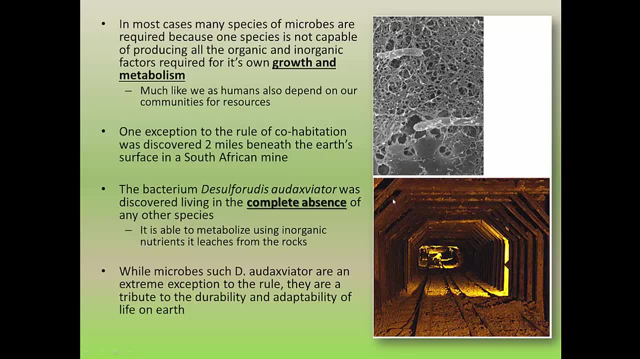 there and were curious about what kind of microbes they would find. so they took samples out of some of the cracks in these coal mines and they were able to find this really unique species that was growing in complete isolation, and so this microbe would be like doing the equivalent of like what I 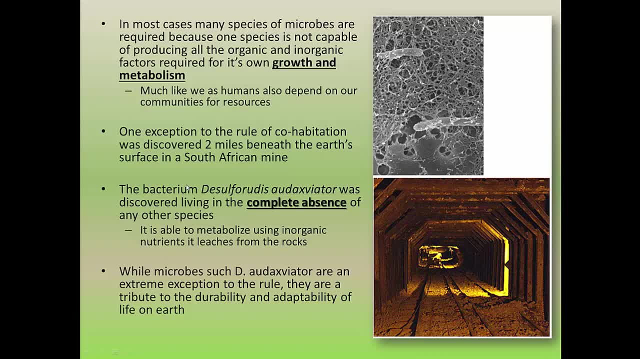 mentioned, where you would have to create all your own food, your own shelter, find your own water, survive against all the elements. this micro basically does everything on its own and, uh, it's pretty a pretty rare thing. life always seems to find a way. there's always exceptions and 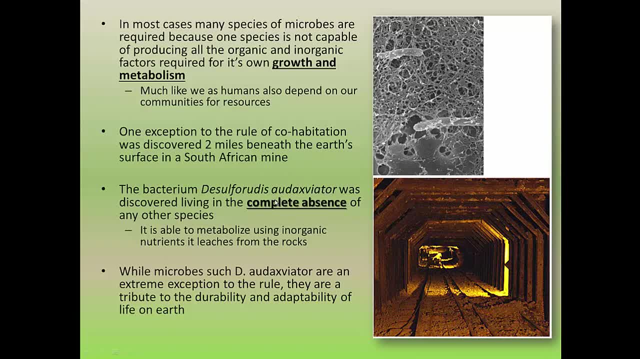 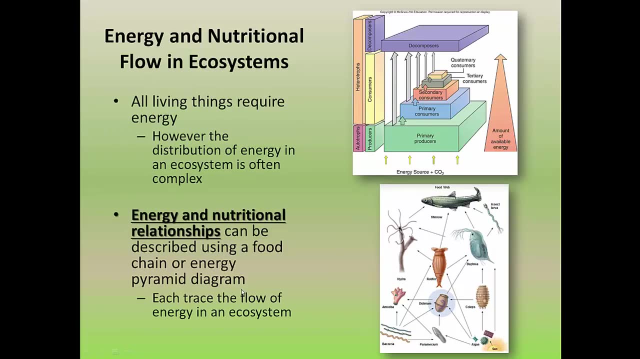 this is one of those where, even even as difficult as that is, there are microbes that get it done. so the species here- certainly a unique type, but anyway- found two miles beneath their surface and cracks in this coal mine. so in most cases you wouldn't find something like that. but 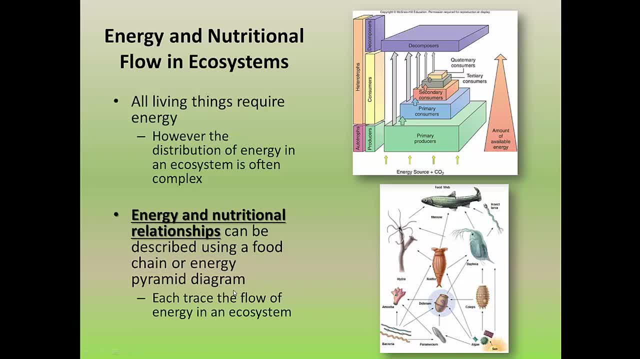 there's always unique species like that. okay, so in the next section, we're going to look at the way energy flows through an ecosystem. now this relates to microbes, as well as all all other living types of organisms, so this is really more of a general ecological concept, one that relates to all types of species. 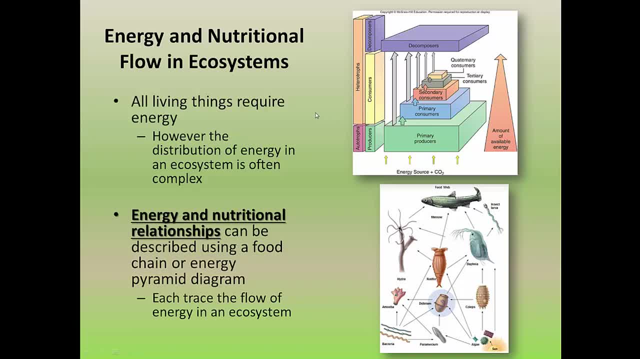 so like to demonstrate this information is to use a figure, as shown here in the top right, that's called an energy pyramid or energy diet, energy pyramid diagrams- what this is referred to as here. we'll talk about this going forward here for the next few slides and then, towards the end, I'll talk about 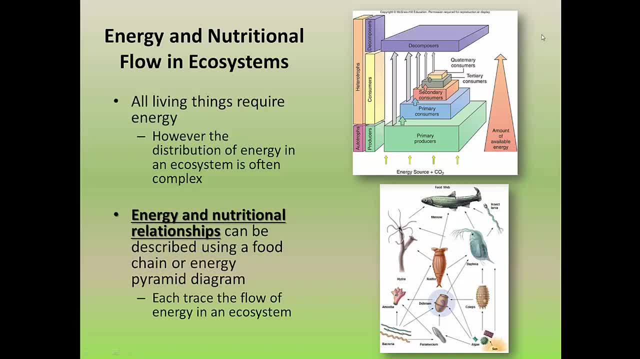 another way to show that which is shown here. it's called a food web. so there's an energy pyramid in a food web and both are showing similar but slightly different aspects of energy and nutritional flow. so we'll start with the food pyramid: what this is showing. 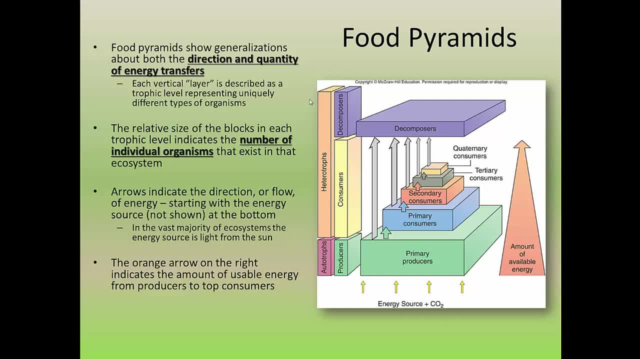 is. it's showing the flow of energy starting from the source and how it very predictably moves from one type of organism to another, and then I'll mention kind of how that cycles back into the environment through one particular group, here called the decomposers. now there's 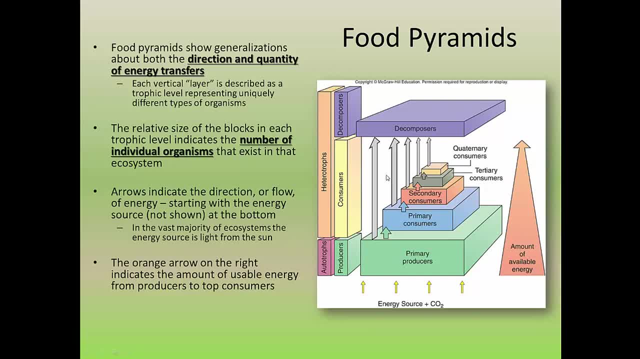 lots of different ways to show this type of food pyramid to figure out of our textbook and, uh, it's- it's a little different than a lot of those I've seen. what I really want to focus on here is this section here and kind of ignore these blocks. 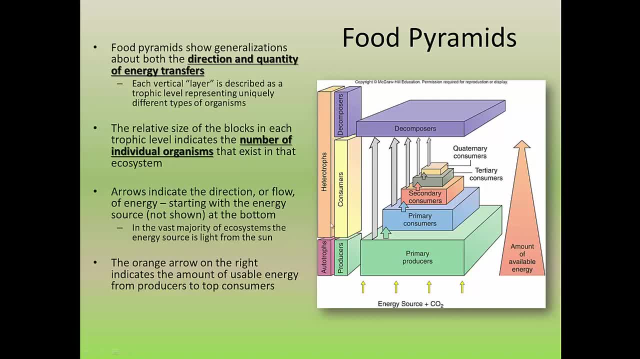 off to the left, those, those are part of it, but for the most part, we don't have to look at those, so we're really going to focus on this section here. okay, that's what I'm going to talk about. so what we typically start by showing is the. 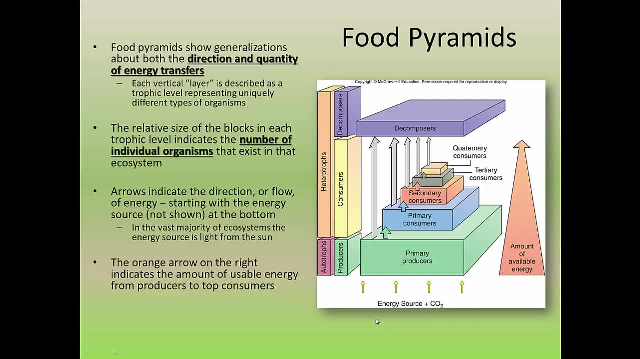 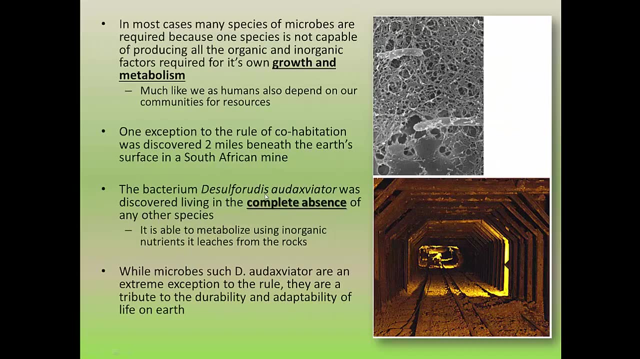 energy source. now, in most cases, that energy source is the sun, so our sun is the primary source of energy, beams down photons and those photons are used to create energy by plants and things like that. there are exceptions in some cases. you know like we go back to this species. 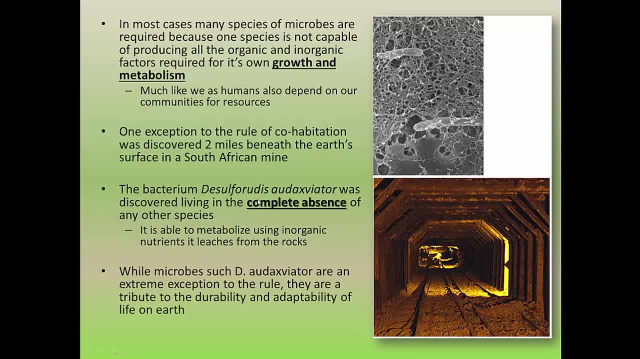 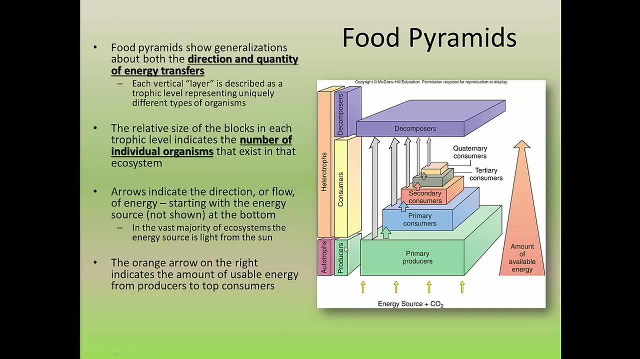 here. this species uses a different energy source, which actually comes from the rocks that it uses in these in the coal mine. so it's two miles beneath the Earth's surface. there is no sunlight down there, so that's why they didn't show the sun here, because 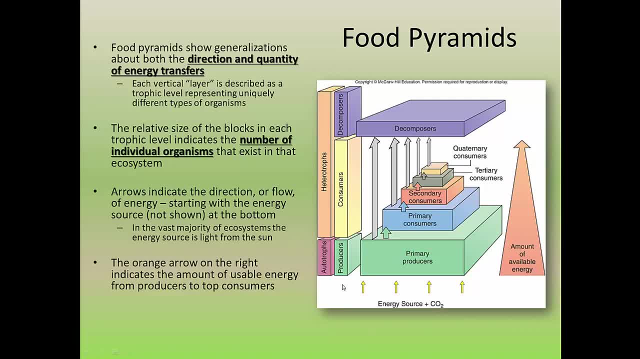 it's not always the energy source, but it's important to recognize that in the vast majority of cases, that is your energy source, with the exceptions being the only time that that wouldn't take place. so the sun is typically the source, and what happens in that case is it beams down? 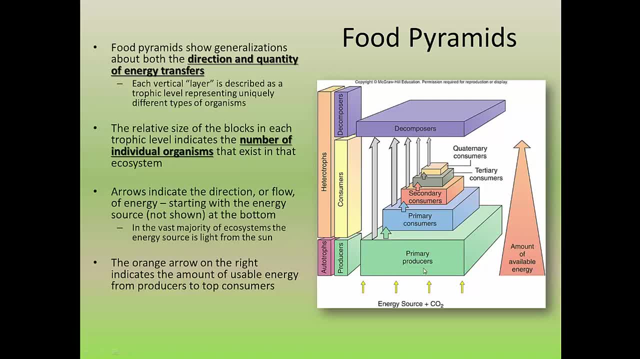 photons that are picked up by our what are called primary producers, so we'll talk about those next here. that's the first organism to grab the energy, and then what happens then is the energy shown by these arrows here is passed from one type of organism to the next. so we see this. 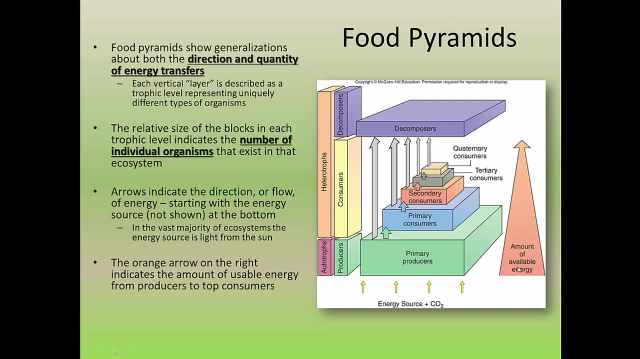 kind of cascade of energy transfer from one to the next here, okay, and that's showing over here as well. now, in addition to the flow of energy, we've also got these arrows over here showing energy. in addition to that, we've also got blocks for each type of species. so primary producers, that's one. 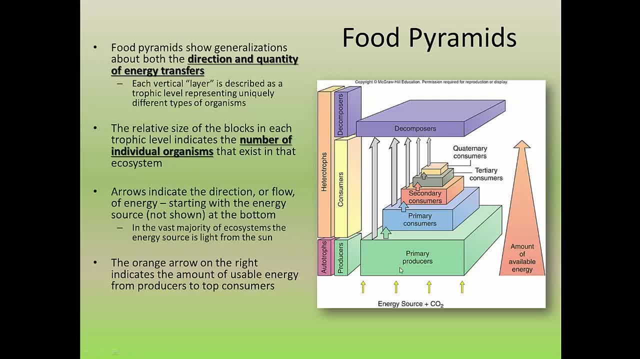 it's not- I shouldn't say- type of species, a type, a broad category of organism based on where they consume energy. so lots of things would fall into that group there, for example. so we show the blocks based on the type of organism and, if you notice, the blocks are: 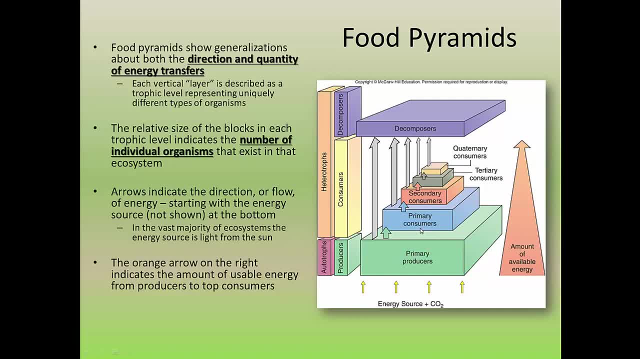 different sizes, starting with the largest, and they get smaller and smaller as you go up. and that's not a coincidence. that's shown by design there. the blocks show the relative size of the populations of each one of these different types of organisms. so how many primary producers? 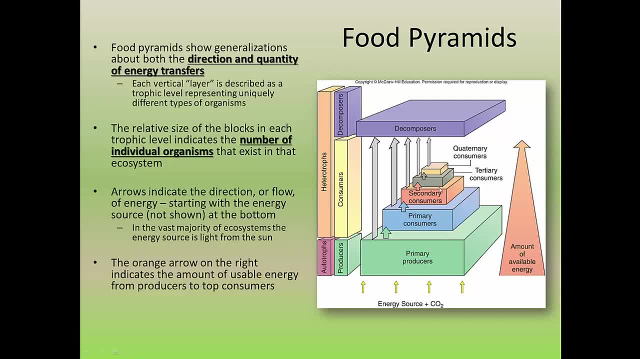 for example, you have in comparison to say, what are called quaternary consumers. so, if you notice, the block is much bigger for the producer than it is for the quaternary consumer. so we'll talk about why that is, but for now I just want to point out that that's what this is showing: energy flow. 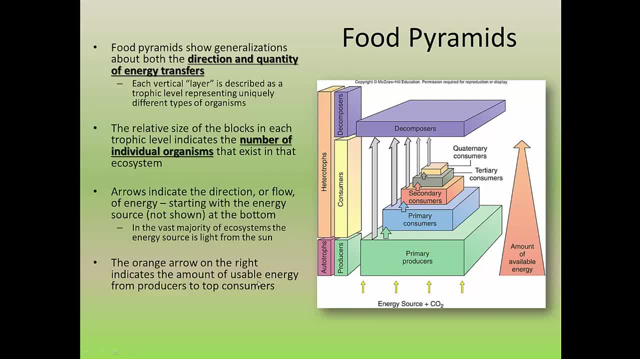 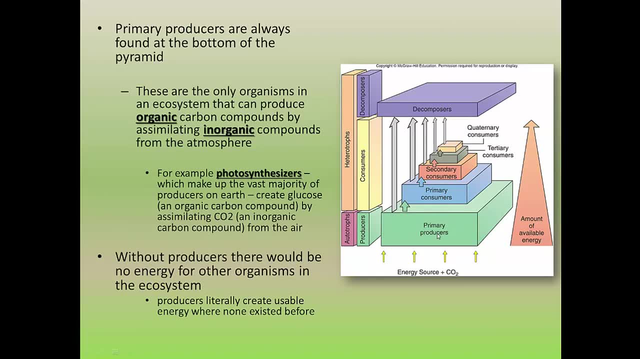 and the relative size of each group of organism here. so, as I mentioned, the primary producers get their energy directly from the energy source, which in this case is the sun, and in most cases where they're getting this from the sun, these are what we call photosynthesizers. so photosynthesizers are the most common type of primary producer. 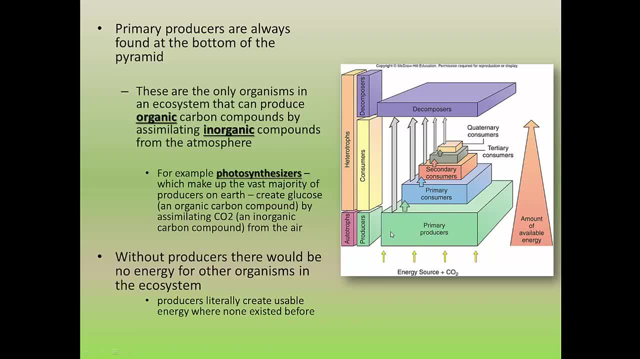 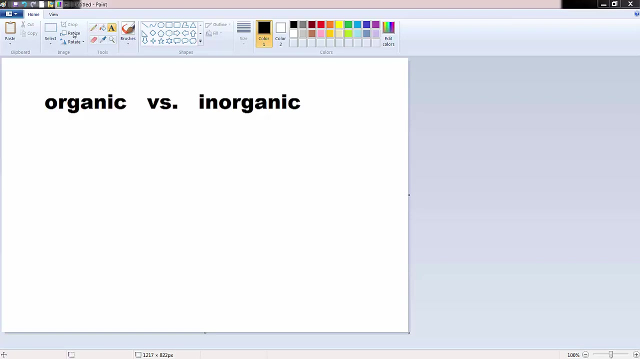 and so these are basically your plants on land and the algae in the water and what they do is they take sunlight and they turn it into food essentially, and a little bit more specifically, they can take inorganic compounds and synthesize organic compounds from them. now, when most people think about organic- the term organic- they think in reference to food organic. 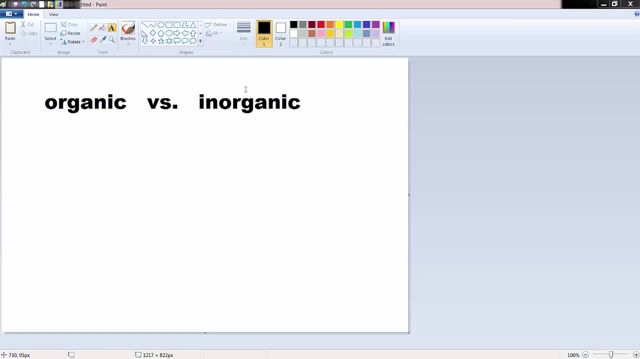 food and they might assume then the inorganic would be like GMO food or food with pesticides in it. that's not really the case there. in this, in these, in this sense of the term, we're actually talking more about the chemical composition of the food. so these terms can apply in a 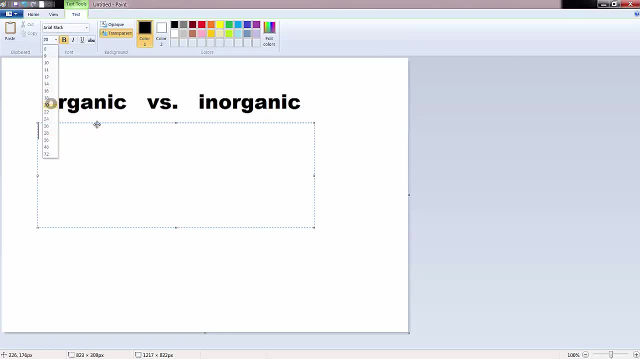 sense of chemistry, talking about the types of elements and chemicals found in them. so, for example, organic chemicals, organic compounds, are actually defined as having combinations. I should say they contain combinations of the elements carbon and hydrogen- carbon C and hydrogen each. so an example would be a common, common type of organic. 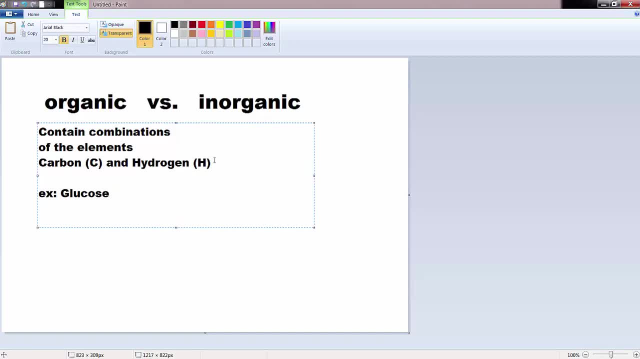 compound called glucose that we'll mention here in a minute, and glucose is made up of six carbons, 12 hydrogens and then also six oxygen. so a organic compound like glucose is defined as being organic because it has the combination of carbon and hydrogen but, to clarify, it can have other elements with it, like oxygen, so long as it. 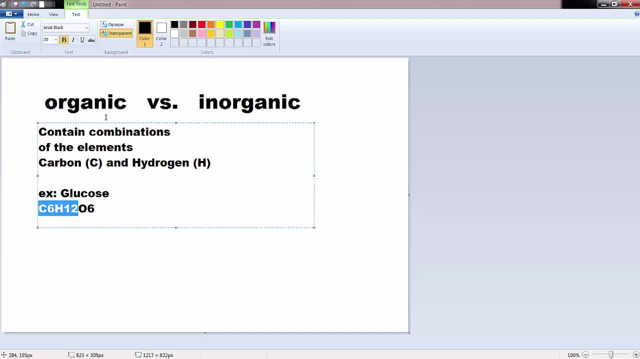 has the two primary elements, carbon and hydrogen, so they contain these combinations and then can also have many variable other types of elements with them. so that's again. glucose is an example. another example that would have just carbon and hydrogen is that it contains carbon, and hydrogen would be a compound like methane. it's one that we'll talk about as well. methane, in this case, is: 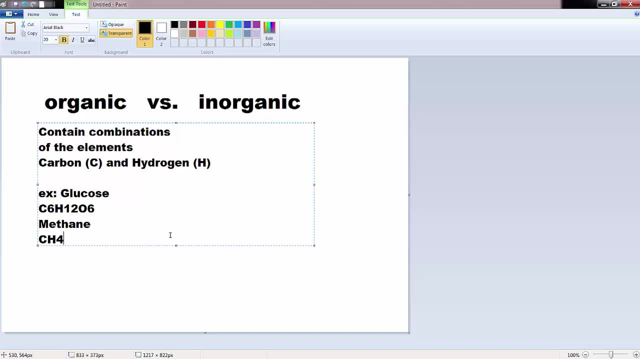 CH4, so one carbon, four hydrogen. so that's also organic, so it can have. you have to have at least these two, and then you can have others on top of that and all those would be considered organic. okay, so inorganic then it's a little more complicated than that, but it's a little more. 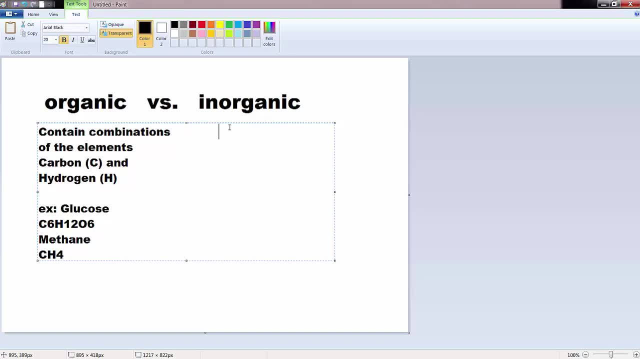 broad and that's basically chemical or chemical compounds that gleich, combinations of lack, combinations of carbon and hydrogen. so these are a little more broad and, and because the definition is a quite specific, there are really many more of these. so an example would be something like carbon dioxide, common component of the air. Another example would be water, H2O. 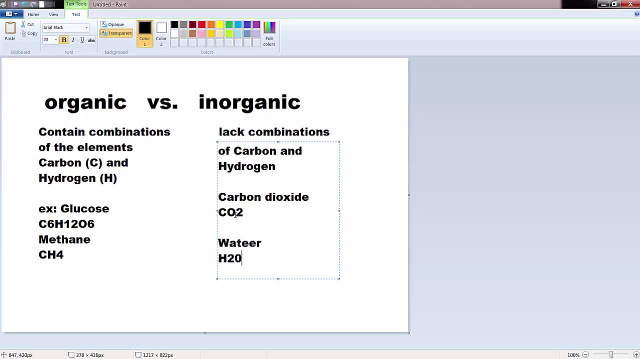 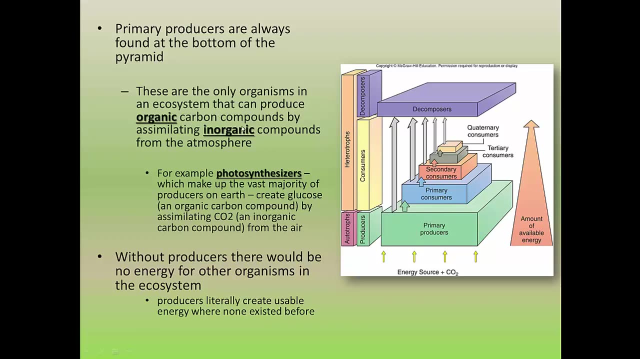 Now, both of these have carbon and hydrogen, but they don't have combinations of them. therefore, they're considered inorganic. Okay, so all sorts of different inorganic compounds out there. So what photosynthesizers do is they actually take inorganic compounds and they convert them into organic. 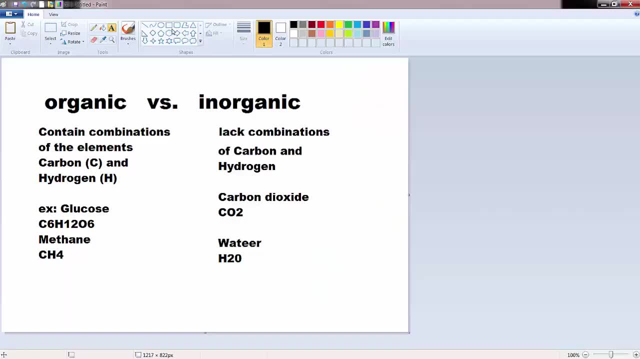 compounds. So one of the reasons why I mention these here is because what photosynthesizers do in particular is they take these two here: carbon, carbon dioxide and water, and they actually convert it into glucose C6H12O6.. So 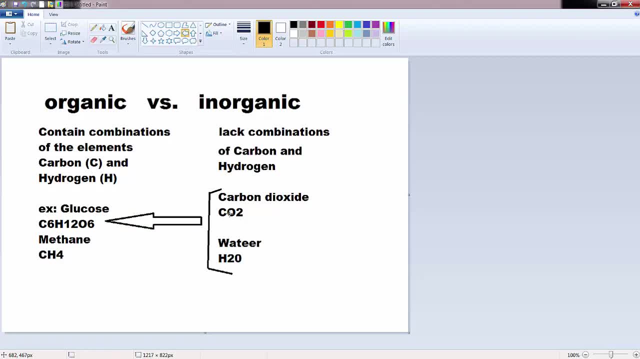 they're basically sucking what would be unusable compounds to all other types of organisms right out of the air and converting it which was a spilled water, and then converting that directly into an organic compound, So they literally make the food that we eat. 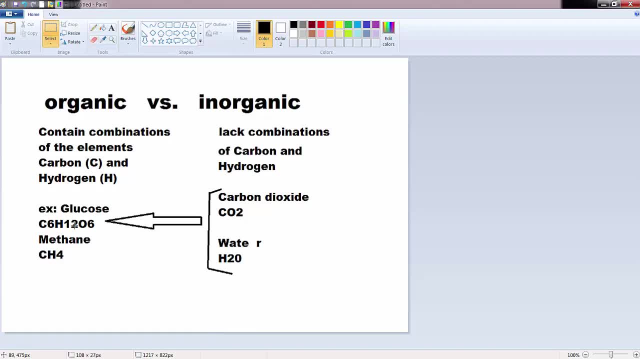 So just to clarify you and I, then we have to consume some kind of organic compound like glucose and fats and proteins. these are all made of different combinations of organic molecules, So really no matter what you're eating. by technical definition of an organic compound, 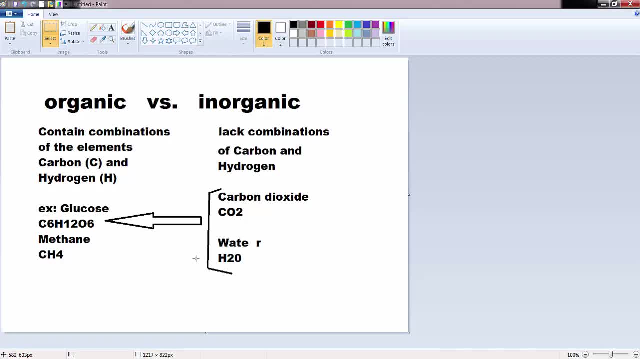 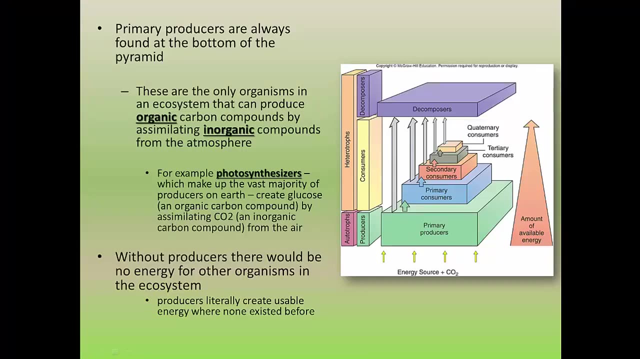 everything that you eat is organic. You really can't digest inorganic compound. That's where there's a different term for organic versus non-organic food. That's when you get into the, the way it was grown and the pesticides and herbicides. That's. that's really a different definition altogether Sounds. 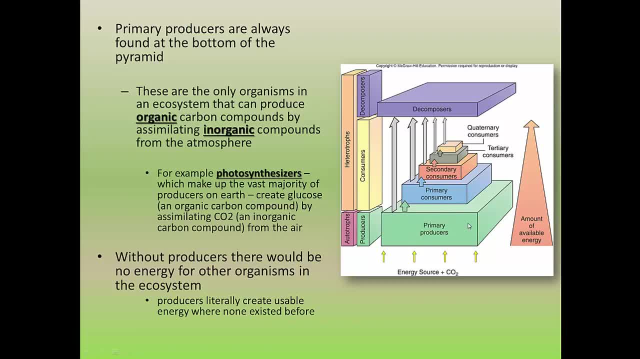 similar, but it's actually not So. in other words, photosynthesizers: they make the food and they use the energy from the sun as part of that process. They can use the CO2,, they can use the water, and the energy from the sun is kind of what. 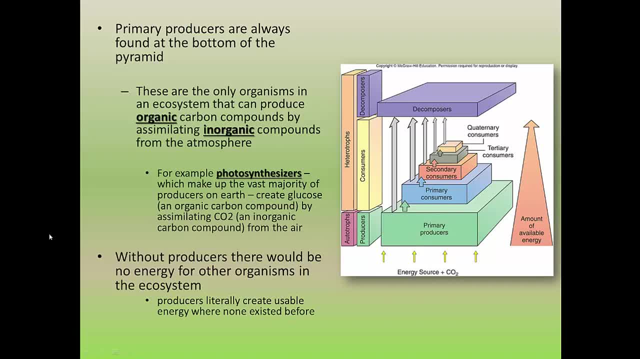 allows them to mix those two together, combine the two together. So without producers we wouldn't have the organic molecules and the energy that other organisms feed off, So they literally create the organic food for other organisms. Now, everything else, then, either feeds directly off the primary 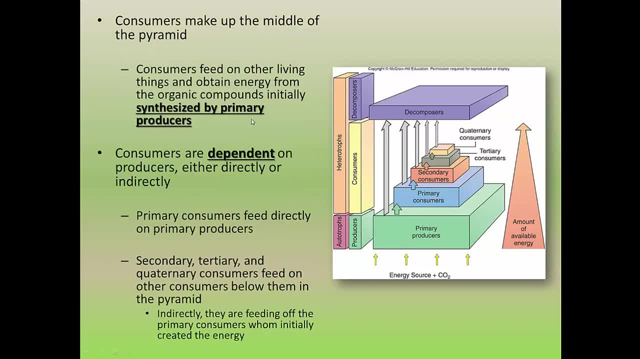 producers or feeds indirectly off of that. So, for example, consumers can be one group- are considered primary consumers? You got primary, secondary, tertiary and quaternary. Primary consumers are those that are defined by feeding directly off the producers. So these are things like herbivores. 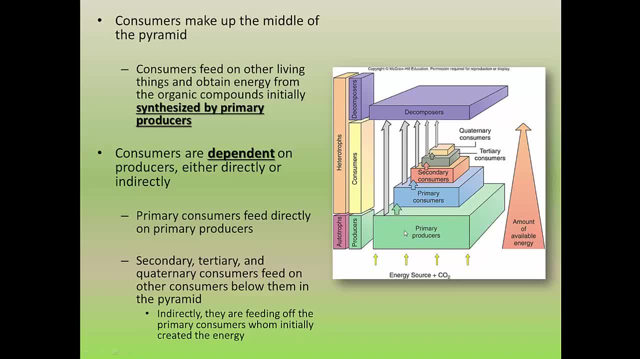 rabbits and squirrels and cows. They feed directly off of plant matter And that makes them a primary consumer, So they're getting their energy directly from the source, which are the primary producers, But, it's important to note, they cannot get energy. 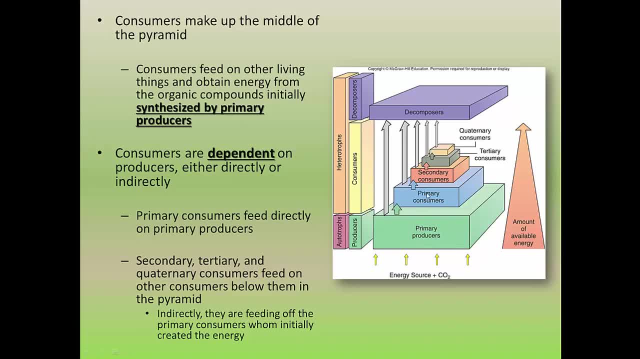 if it's not given to them via producers. So they are dependent on the energy they get from the sun. Now, a secondary consumer is an organism that would feed off the primary consumers. So these are organisms that get their energy indirectly from the primary producers. 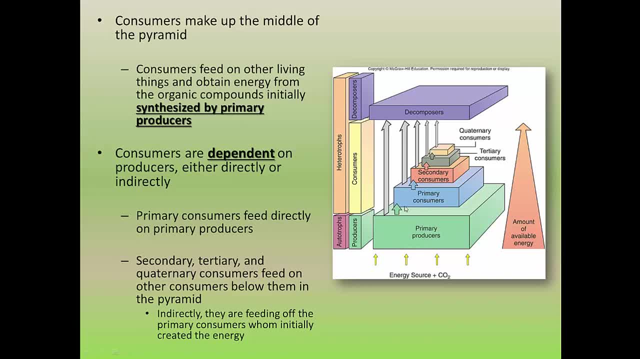 So in order for them to get energy, it has to go first to the producers, then to the consumers, and then to the primary consumers and then to the secondary consumers. Tertiary consumers feed off the secondary consumer and quaternary consumers feed off of the tertiary consumer. 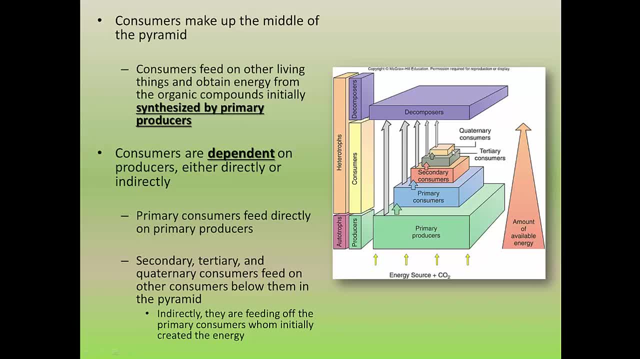 Now you can. in some every ecosystem is different. Usually you don't show it past this point because it kind of just illustrates the overall concept. But to be fair, you could have additional levels of consumers after that. So the idea is every group feeds on the group below it. 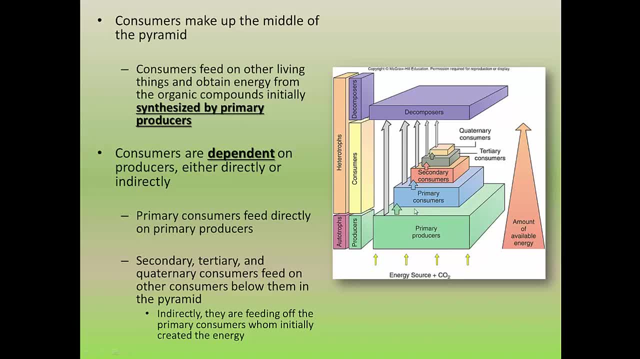 Now, as I'll mention towards the end, this is somewhat of a simplified version of reality. The truth is, there's lots of organisms. Take like pigs, for example. Pigs will pretty much eat anything that you give them, literally, So they could feed off plant matter like corn. 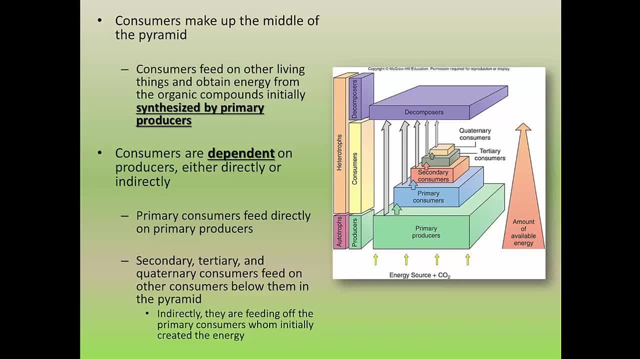 or they could eat living things. Pigs have been known to eat people. unfortunately, If you fall down in a you know a pig cage, a pig pen, people have been known to be eaten unfortunately, So things like that would be a group. 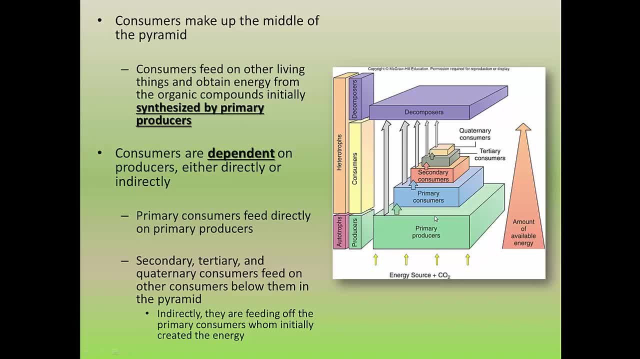 an organism that wouldn't fit so neatly into this diagram, But the idea is that it shows a concept as opposed to an absolute set of examples that work in every scenario, And that's where the last slide here, in part one, comes in. That'll be what's called the food web. 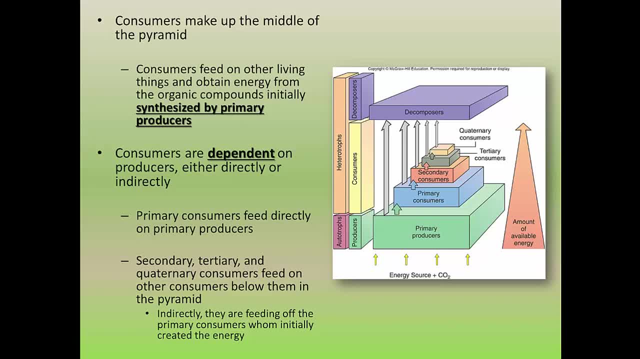 is designed to show a little bit more of an accurate, specific set of energy transfers that you would use for each particular environment or ecosystem. So this is more of a concept as opposed to an absolute. But that is how it generally works. One type of organism feeds off the next. 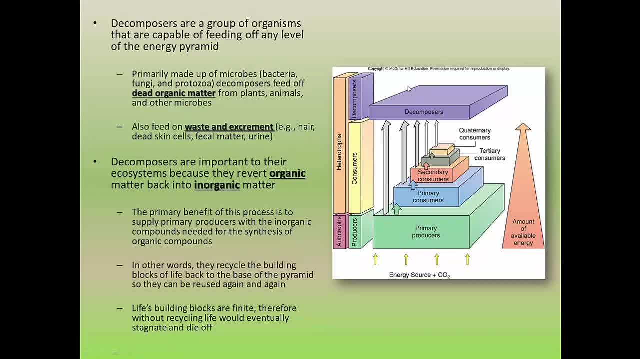 Now, at the very top up here, they've shown another really important group of organisms, referred to as the decomposers. So decomposers are shown separate from the other levels And they're also being shown with a separate set of arrows going up to them, so that what this is showing 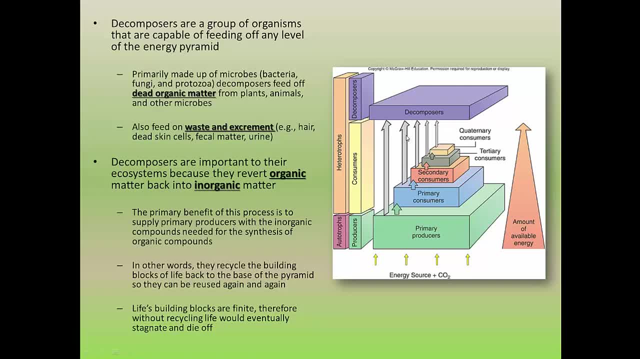 is energy from any level can be transferred to the decomposers separate from the energy transferred from one level to the next, And the reason for that is that decomposers will simply feed on any of the dead remains or the waste that is given off. 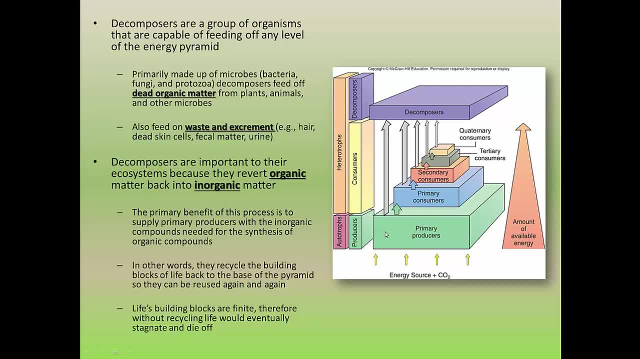 by any type of organism. So if a plant dies, like a tree falls over and dies, things like fungi will feed off of the bark and the dead organic matter of the tree, usually over many years, and break that down very slowly. So they will feed off of the dead organic matter of the tree. 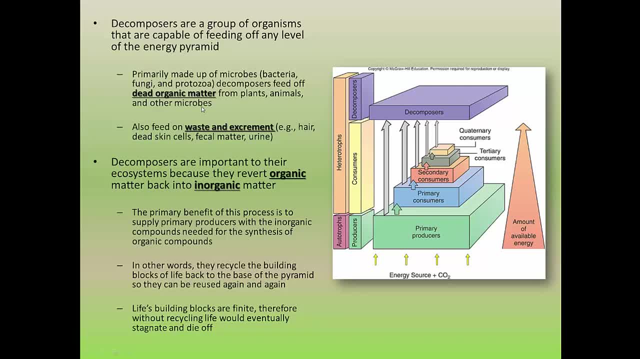 They'll also feed off the waste leaves that fall every fall. Those are an example of a waste product- dead skin cells for humans- So fungi and bacteria can also feed off of that as well. Also things like hair, dead skin cells, fecal matter, urine. 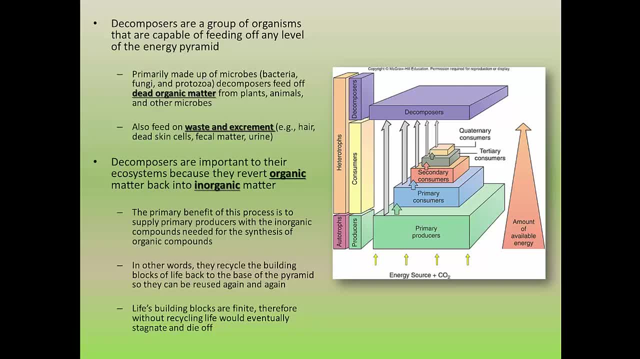 all these things are consumed by a wide variety of different types of organisms, as well as insects, even certain types of birds like buzzards. They feed off of dead carcasses, and all sorts of things will feed off of dead animals and dead remains. 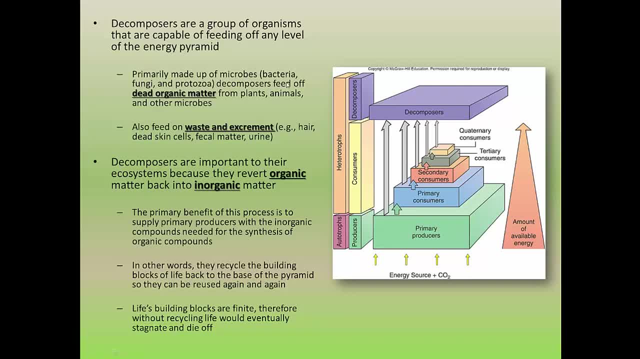 So decomposers are actually a fairly wide variety of organisms, But from a microbial stance, most of them are things like bacteria, fungi and even protozoa. But the idea is that they don't really fall into the flow like the rest of these organisms. 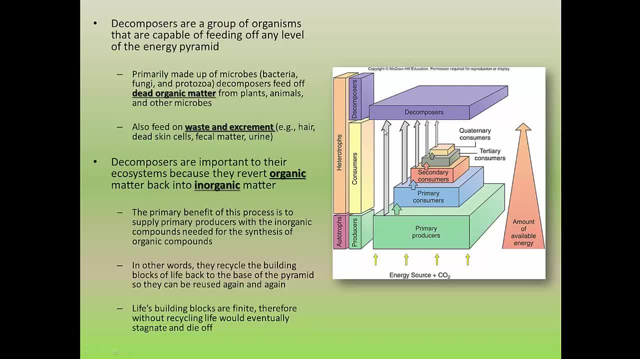 That's why they're shown off to the side here. They just pretty much feed off anything that gives them a source in reference to waste and dead remains. Now, one of the things why they're important is that decomposers are key to recycling. 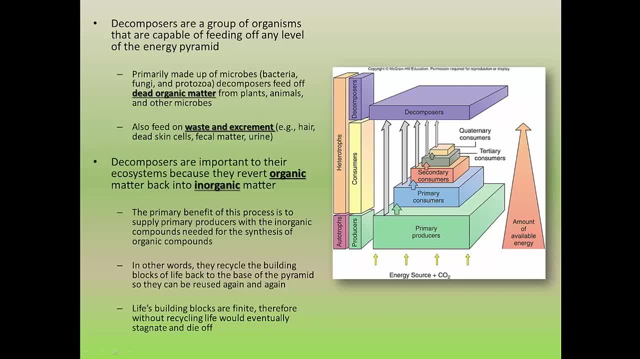 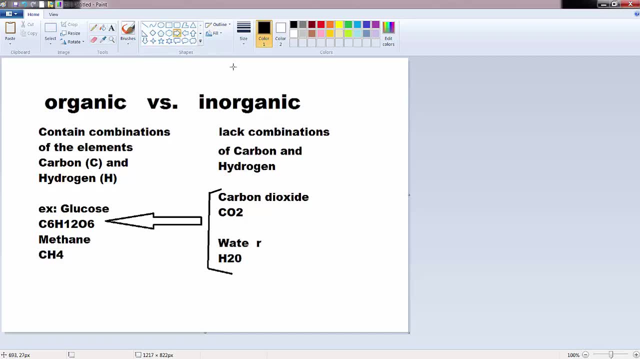 some of the organic matter back into inorganic matter. Now, they're not the only organisms that do this, So they're not exclusively the only types that do this, But they are. They are key to taking certain forms of organic matter in particular and reverting that back. 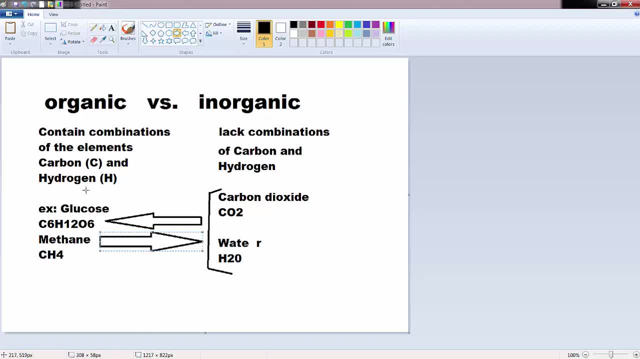 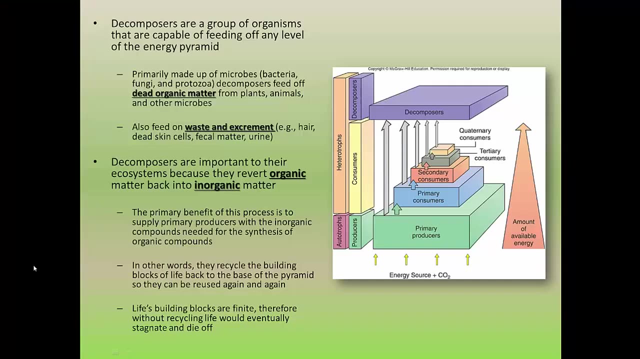 into the inorganic building blocks. So what that does? it allows a cycle of both inorganic and inorganic chemicals to be fluctuating back and forth at all times, So it makes this whole process cyclic. And without them, what would end up happening is you would start. 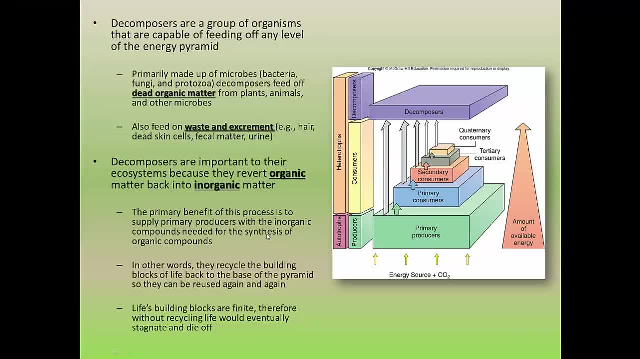 to run out, Run out of some of the inorganic building blocks, or they would at least start to become limited, And, as a result, producers would have a hard time creating as many organic compounds because they'd be limited on the building blocks to make those. 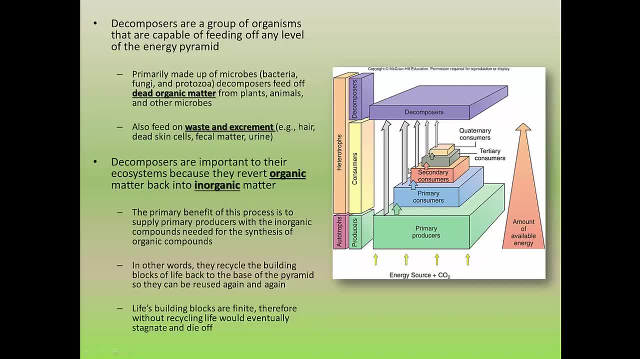 So the decomposers are important for taking what organic compounds exist within these groups and returning them back to a form like CO2, so that you have a new source for organisms to utilize. Now CO2 is actually kind of a bad example, Because you and I, as consumers, we give off CO2. 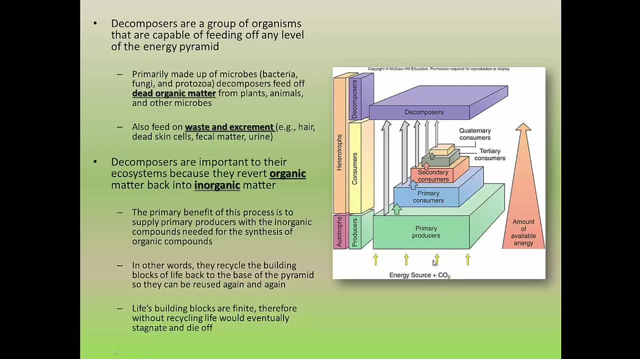 when we breathe, to be fair. So they're not as important for things like CO2, more important for things like nitrogen and phosphorus and sulfur, calcium and things like that. So we'll talk about those in part two, in a little more. 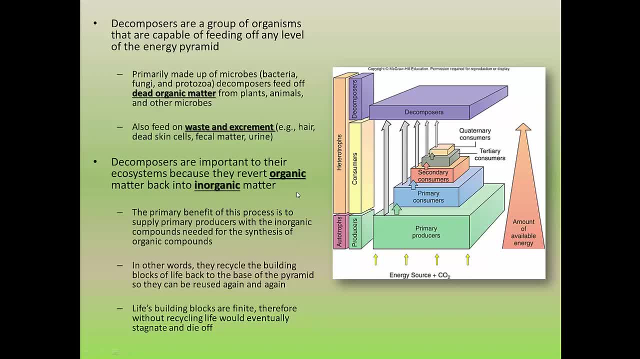 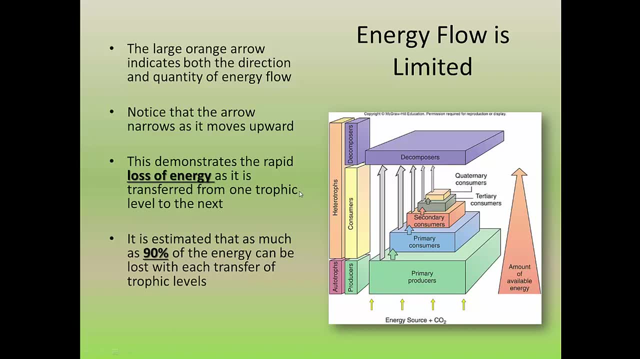 detail, but that's kind of the idea. They return certain inorganic building blocks in particular, back to the environment. So that's why decomposers are important. One of the last things here: energy flow is limited. What that means is that every time energy is consumed, 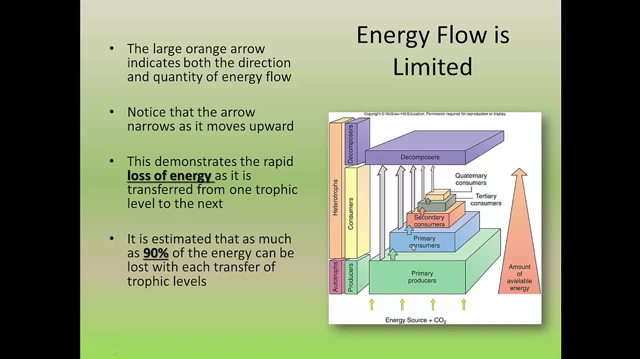 some of it is lost. So, for example, when a primary consumer feeds off of a primary producer, less than 100% of the energy available is actually transferred to the consumer, And this is due really to two reasons. I'll mention them on the next slide. 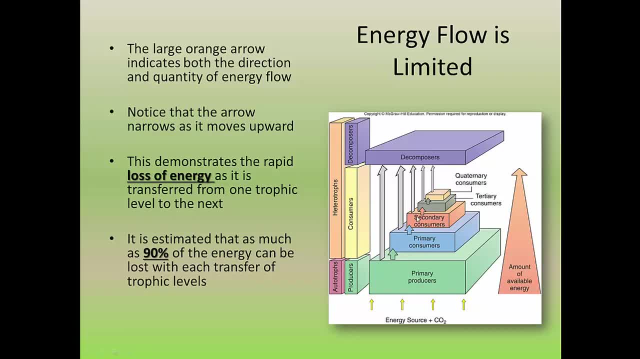 But basically in a nutshell, with every level we move up, these are called trophic levels. Trophic is a reference to energy. Trophic level is mentioned here. So with every transfer of energy from one trophic level, 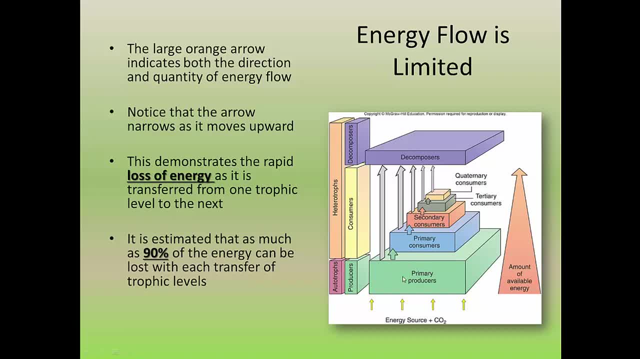 to the next, such as, say, a cow eating the grass, some of the energy in that grass is lost And therefore the cow could never actually absorb 100% of the energy it actually consumes. This is true for you and I. Let's say, you put a cheeseburger. 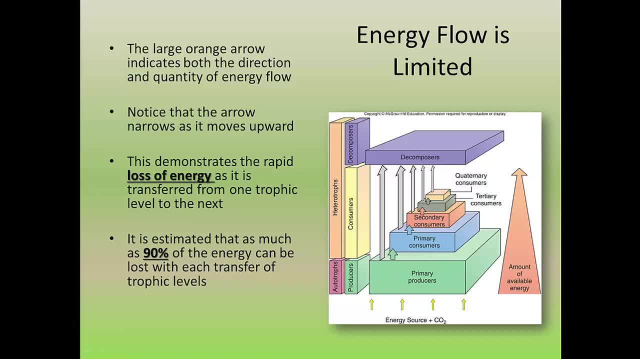 in your body with exactly 1,000 calories. The truth is, your body won't absorb all 1,000 calories. It might feel like it the next day, But you haven't actually absorbed into your physical body all of those calories. 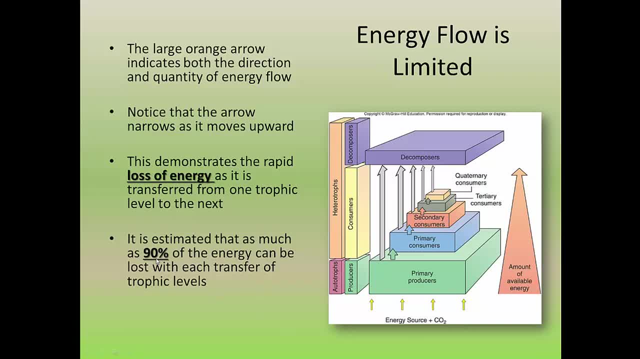 And there's in some cases as much as a 90% loss of energy. It's not always that high, But in some cases it is. In some cases it can be that high. We might wish it was that high with the cheeseburger. 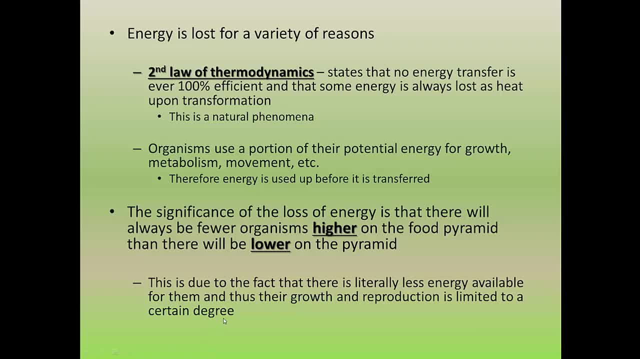 But it is variable. So in some cases you absorb more, In some cases you absorb less. This is also somewhat genetic. There are different metabolic factors that will change that, But the biggest reason why this is is actually a law of nature, a natural phenomenon. 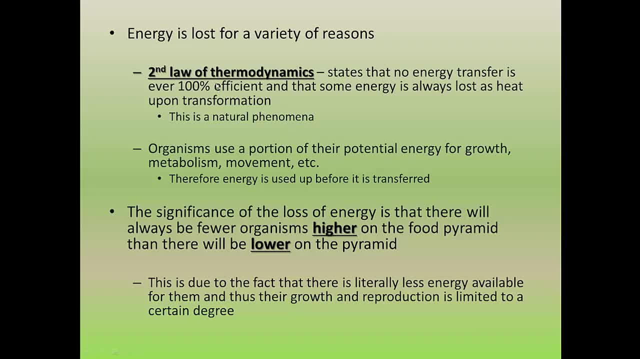 It's referred to as the second law of thermodynamics. So the laws of thermodynamics are related to physics and the way Energy and matter work, And the second law is a very important one And it states that no energy transfer is ever 100% efficient. 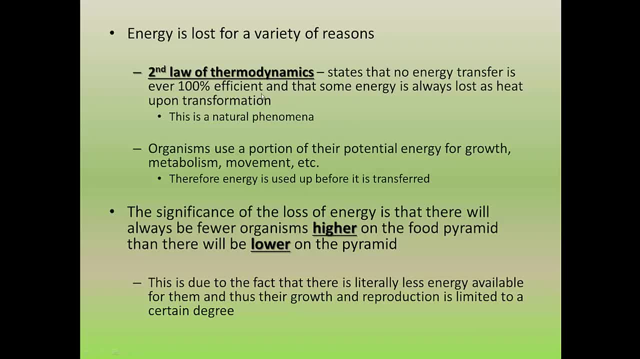 And that some energy is always lost as heat upon transformation. So whenever we eat something, or any time something is consumed, some of the energy is actually lost in the form of heat, And this is something that helps keep our body temperature up. So our bodies have actually adapted. 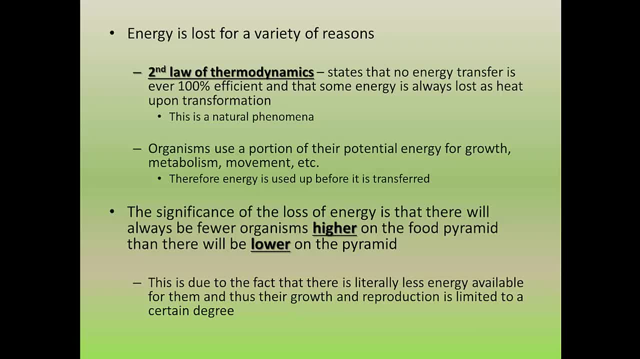 to use that heat energy. But really, what's happening? What's happening there is, the energy is not being used for our body processes And therefore it represents a loss of overall energy. Now, if you go back to this figure here, 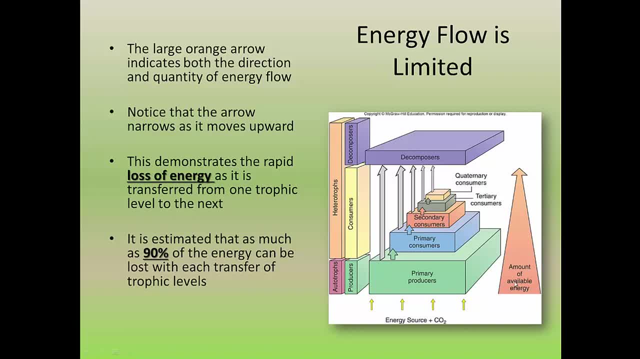 it's showing on this arrow over here on the right, the amount of energy at the base is higher, And as it moves up, the energy narrows, meaning that the amount of energy is less, And so what we're seeing is that the producers, they start out. 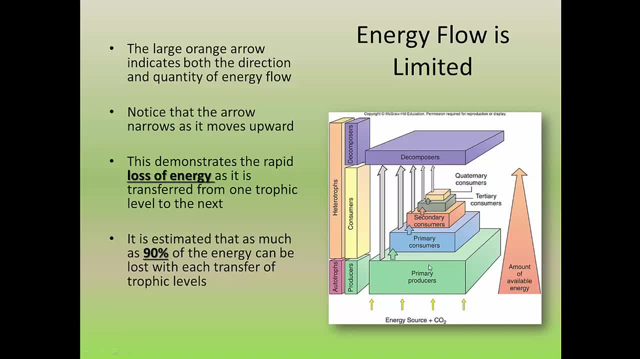 with 100% of the available energy, And so what we're seeing is that the producers, they start out with 100% of the available energy. So 100% of the energy is whatever the primary producers are able to make from the sunlight. 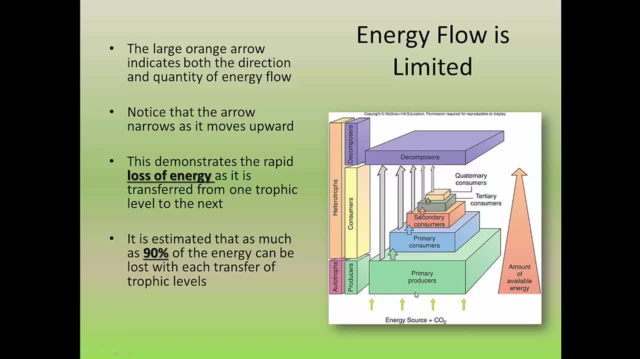 So within any ecosystem, all the available energy is represented by the biomass of your producers. OK, And they're able to get whatever they can from the sun. From that point forward, starting with the primary consumers, they may only absorb 10%, 20%, maybe 30% of the energy. 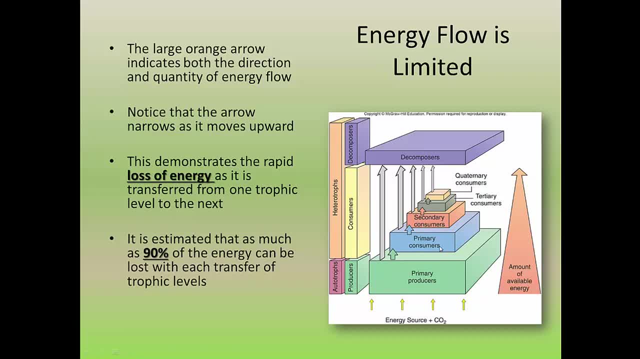 And, as a result, the size of that group of organisms is automatically limited. So the population of any primary consumer will always be a fraction of that, in terms of biomass, compared to the primary producers. Now, in terms of numbers, the numbers. 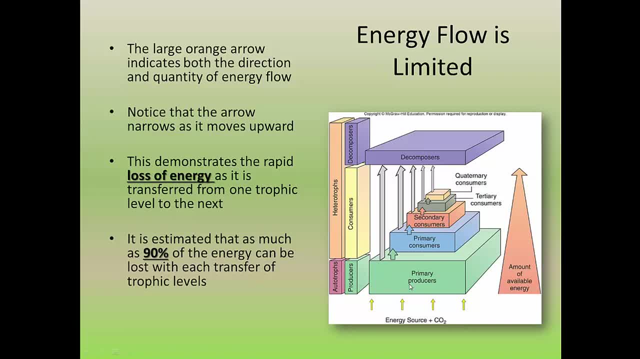 may look a little different. So really the best way to think about it is in terms of biomass, a unit of grams, for example. So there's always less biomass of primary consumers, And then that follows on to the secondary consumers. The same thing happens again. 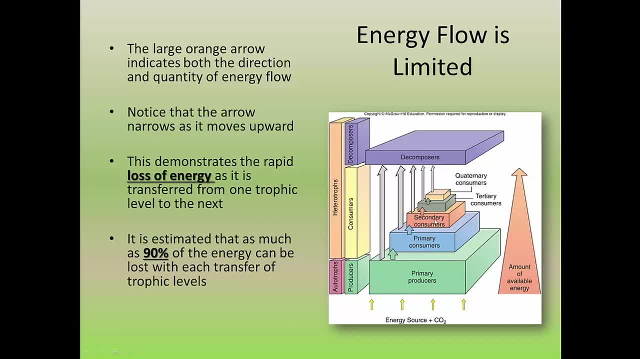 So now even more energy is lost when the secondary consumers feed off the primary consumers, and so on and so forth. So every time we move up a level, a huge amount of energy- up to 90%- is lost And, as a result, the population of each group of organisms. 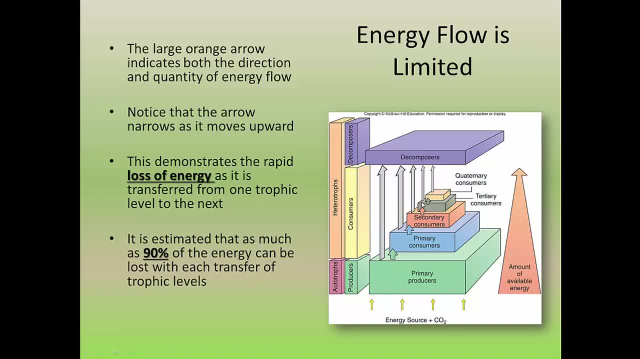 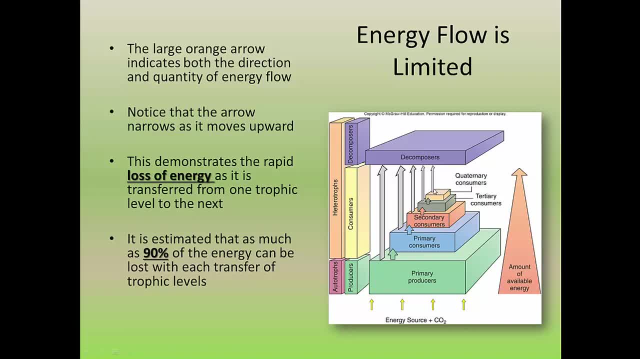 In a prairie grass ecosystem like Kansas, these might be things like coyotes. a fox, These might be predatory birds like owls, hawks. They usually are towards the top of the food chain, if not the very top, And there's always less of those than there. 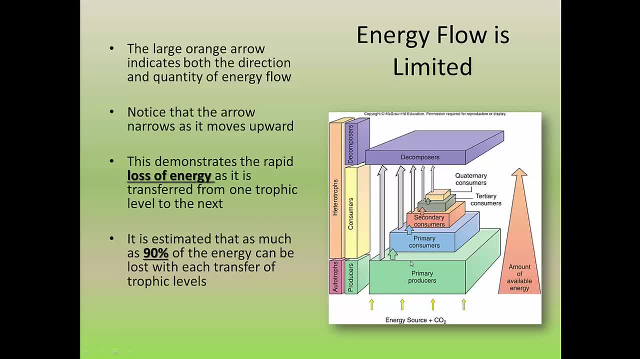 are things like mice. So if you actually look at the amount of biomass that they feed upon, or the grass or the trees or the brush that those organisms feed on, so if you actually were to calculate the amount of biomass, you would find that there would be exponentially more biomass. 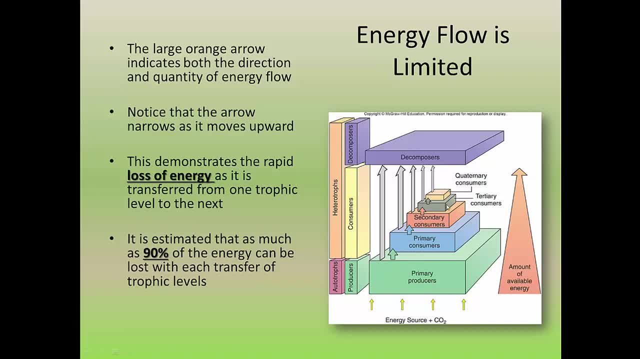 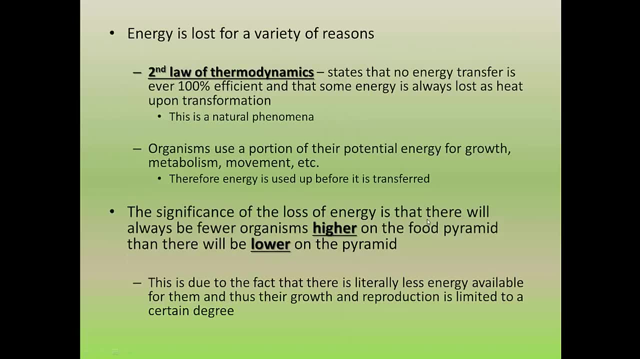 in the trees and in the grass and then the brush, than there would be compared to, say, the hawks and the owls and the coyotes and things like that. So, due to physical limitations of nature, the populations always get smaller, And the only time you have an exception to that, 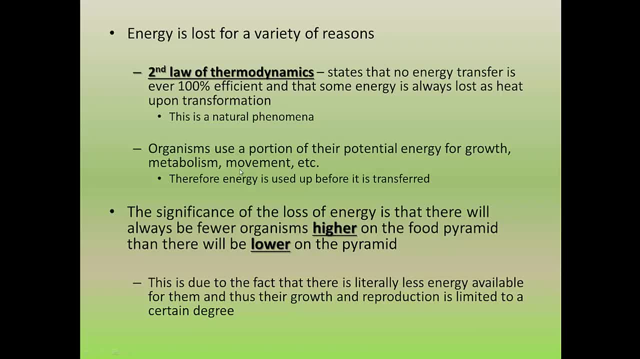 is if there's an imbalance in an ecosystem. So for temporary periods of time, it is possible for higher-level consumers to be equal to, or maybe even slightly outstripped, or become more populous than the previous group, but that would always be temporary. 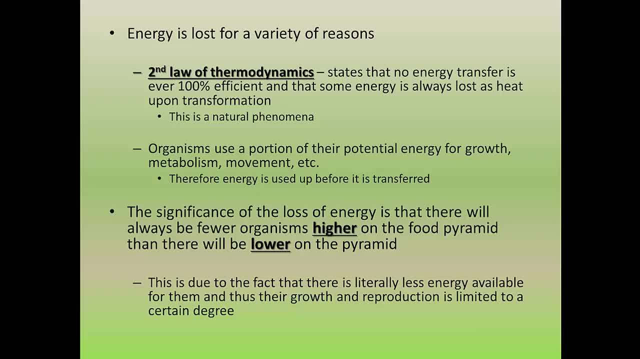 It wouldn't be sustainable. So within a relatively short period of time, the population above would crash back down below. So the only exception to that is if there's an imbalance in an ecosystem, And the only exception to that would be if you had a temporary imbalance in an ecosystem. 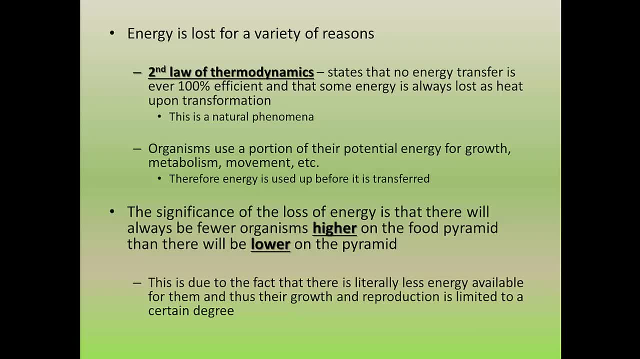 which does happen, and that would not be something that's sustainable. So from a long-term sustainable standpoint, the populations above are always less than those below, So a lot of that has to do with the second law of thermodynamics. The other reason is that organisms are using the energy. 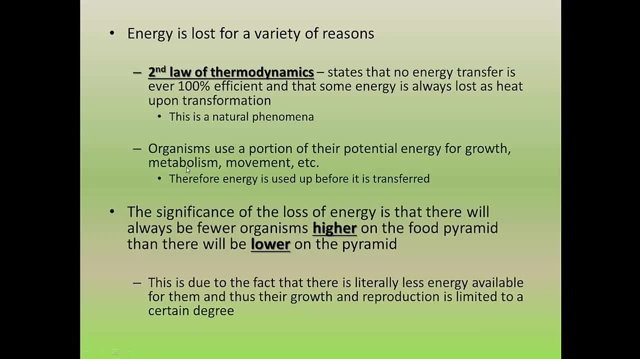 before it's being transferred. So the plants, for example. they don't just suck up energy from the sun and then wait until something eats them. The plants are using that energy- The primary consumers- before they're eaten. they're using that energy as well. 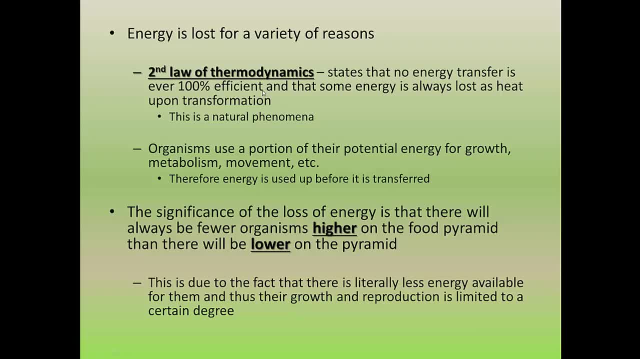 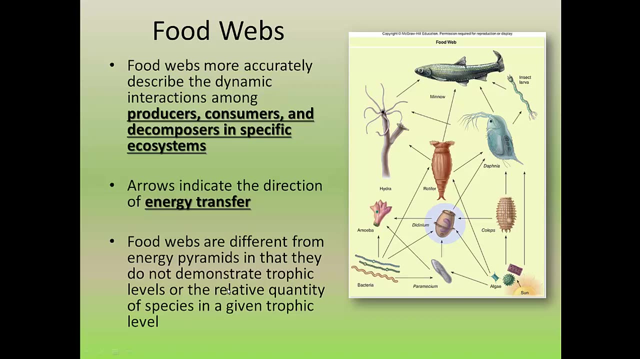 So you'll never absorb. even if you could absorb all of it, there would always be some of it that's lost due to utilization before it gets transferred. Okay, so that's why we have a loss of energy and why we have lower population sizes. 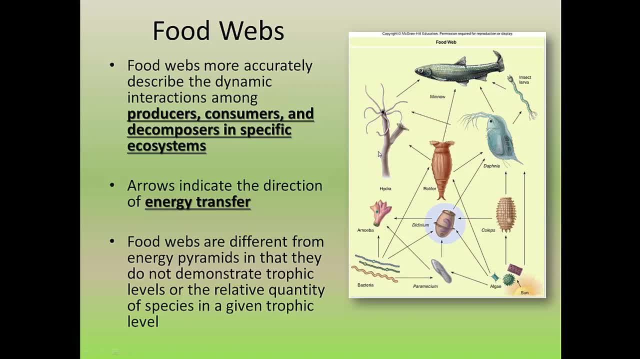 The last slide here is in reference to a more accurate way of showing energy transfer. So this is what we refer to as a food web. So, as I mentioned things like pigs, they don't really fall so neatly into a consumer category. A lot of organisms are like this. 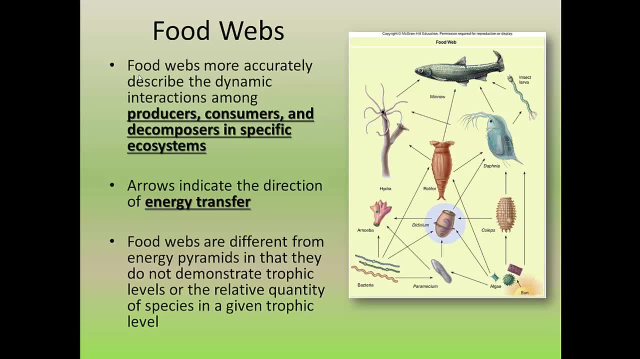 Humans are another one. You know humans were an exception to pretty much every rule. But really, if you want to get more particular and show exactly how energy transfers work in a certain environment, you would use what's called a food web, And a food web is designed to show. 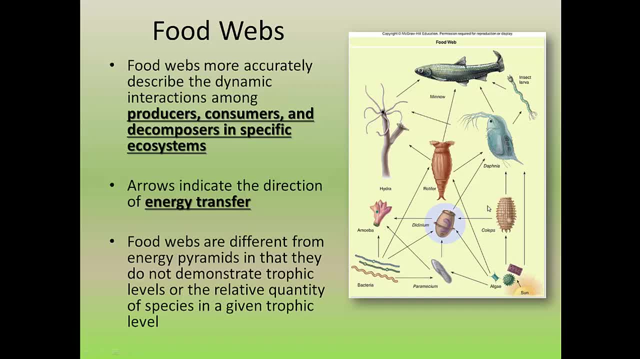 the particular species and how they feed from one source to another. So this is one off an aquatic food web taken right out of the textbook. It shows the source of energy down here being the sun. The primary producers in this case are the algae. 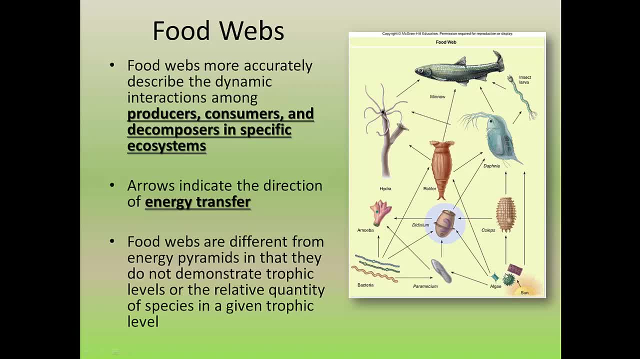 And the algae then. but the arrow, by the way, shows where the energy is being transferred to. So if you actually go backwards, that means that this organism is eating the one before it. So the reverse of the arrow would be: it's eating what? 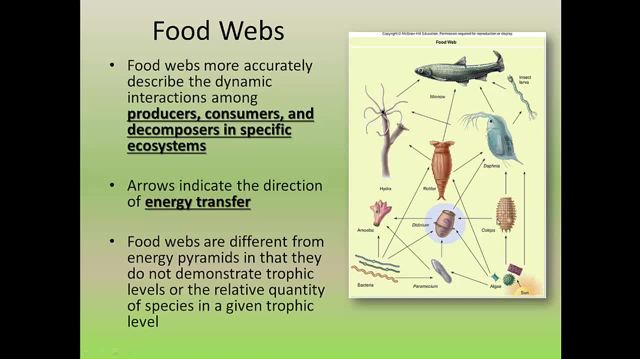 So when we show algae with the arrow going to this thing here called the colops, that means the colops is actually eating the algae. Same here with the diadenium: It's eating the algae. Okay, so the energy is being transferred in that direction. 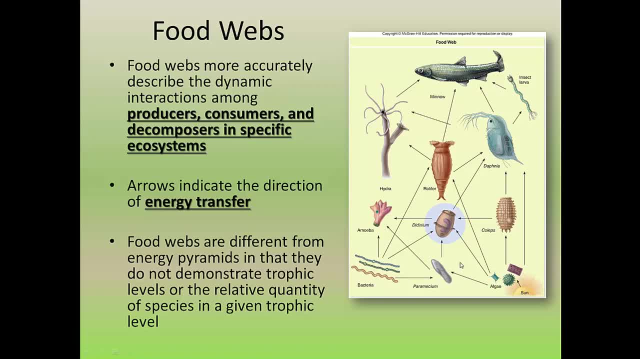 So it's a little more accurate, because the truth is, lots of things feed off lots of other things, And so it gives you a better idea of just how that energy transfer takes place. It's a little harder then to show which is the primary consumer. 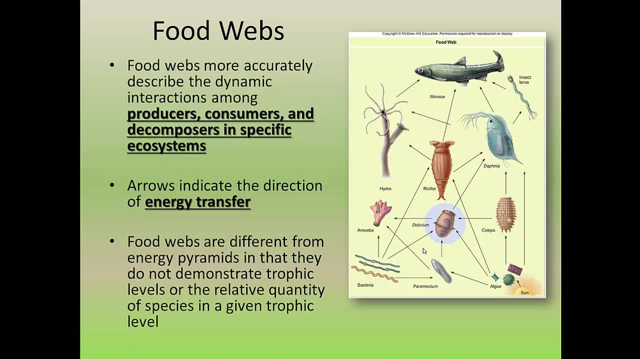 which is the primary or secondary consumer, And the reality is those types of labels aren't quite so easy to identify in truth. So the food pyramid is more of a concept of energy transfer and the food web is more of a realistic rendition of how energy is actually specifically transferred. 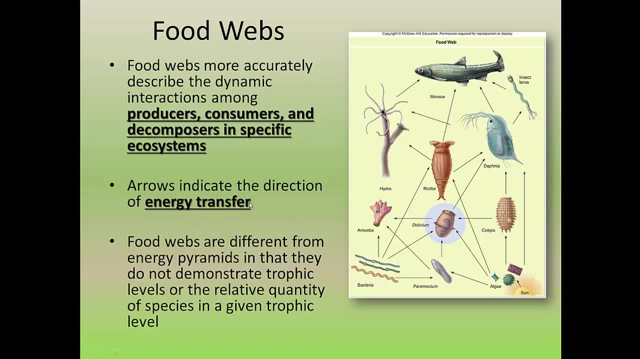 in any particular environment, And that's one of the big differences there between those two. Okay, we'll stop here and we'll pick up start part two next. Thank you.